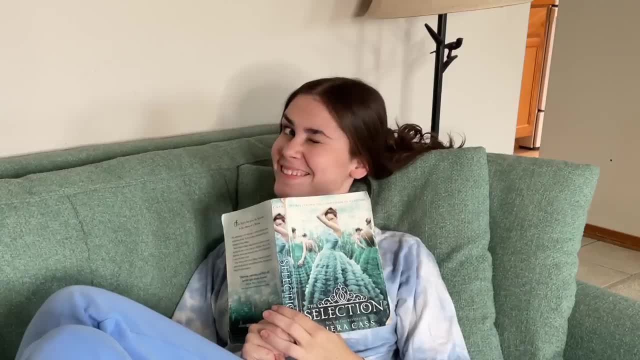 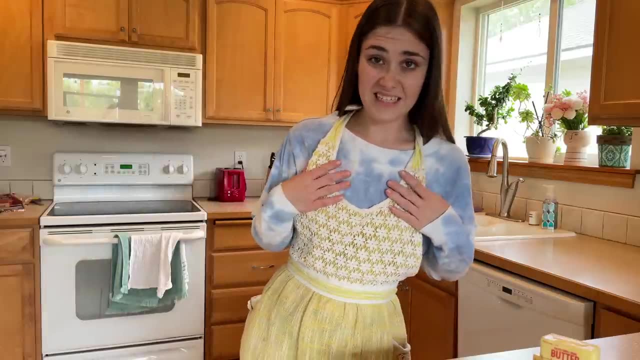 Maybe you like to read and you want to recreate your favorite book cover. Not that I did that or anything. Maybe you're in charge of a last-minute bake sale and you're in dire need of an apron. I didn't actually make this. 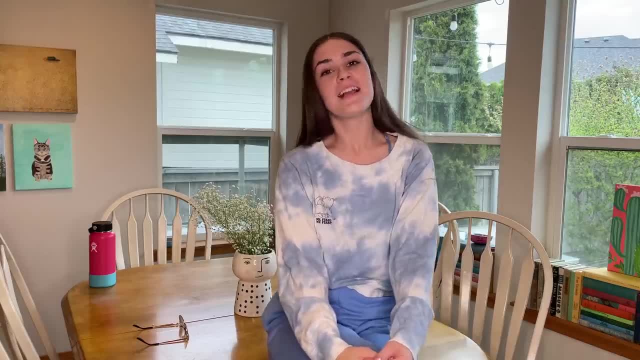 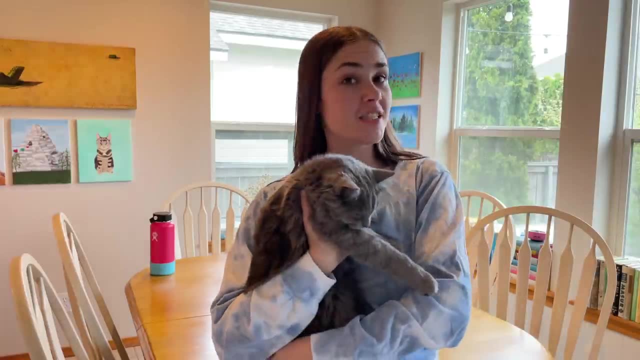 Whatever the case may be, today I have a video showing you exactly what I did to start sewing, and I want to teach you how you can start sewing as well. Before we get started, don't forget to like this video and subscribe, if you haven't already. 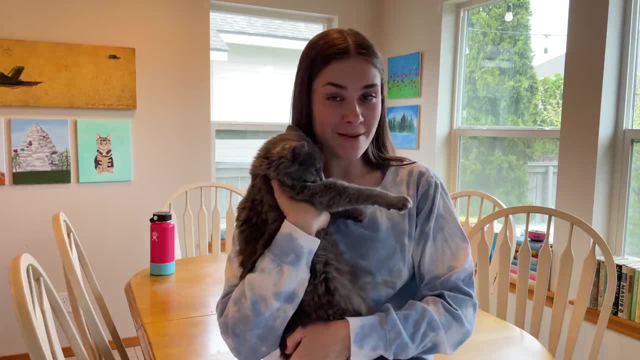 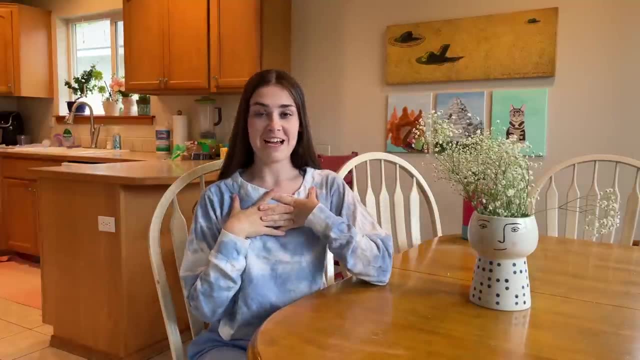 because we have a lot of fun on my channel and I love to share all the things I make with everybody else. Also, say hi to Mabel. Before I start, I want to answer a few questions about myself that I get all of the time. 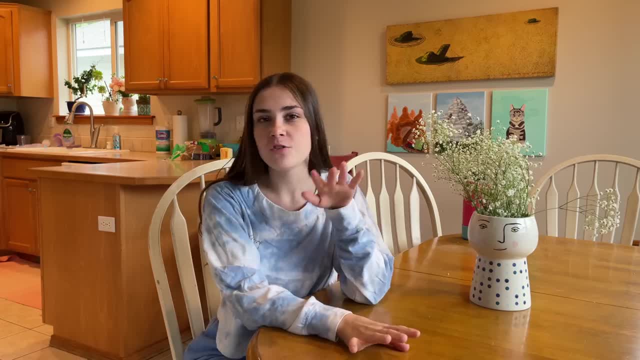 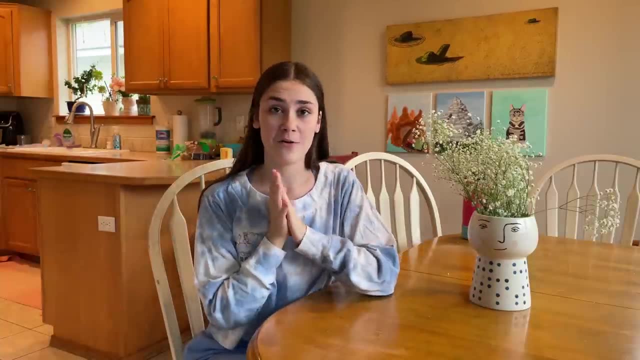 I started sewing in the beginning of quarantine, June, July 2020.. And before I made my first dress, I had never touched a sewing machine. I did not know how to work one at all. I promise I'm not lying to you. 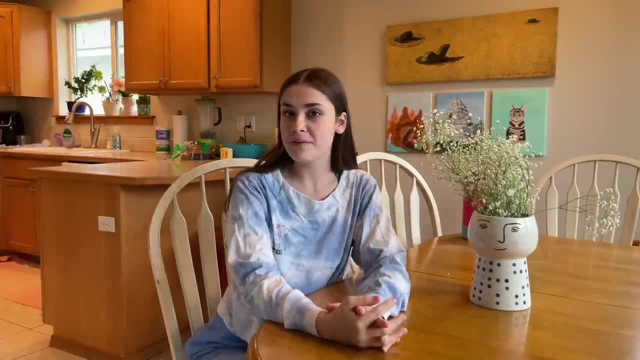 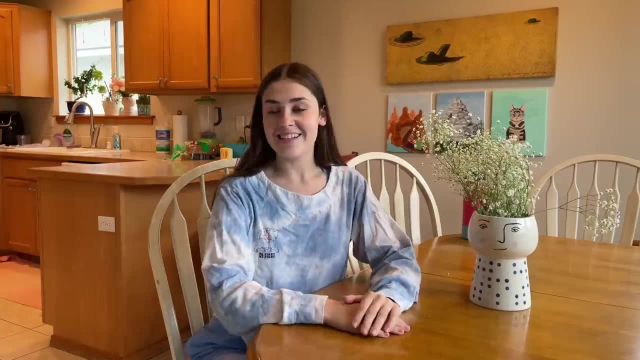 It was all new to me. I, like everybody else, was probably a little bit bored and I was just learning something fun, and I had already gone through a lot of different things. I mean, I even painted a wall mural- And so I decided to start sewing. 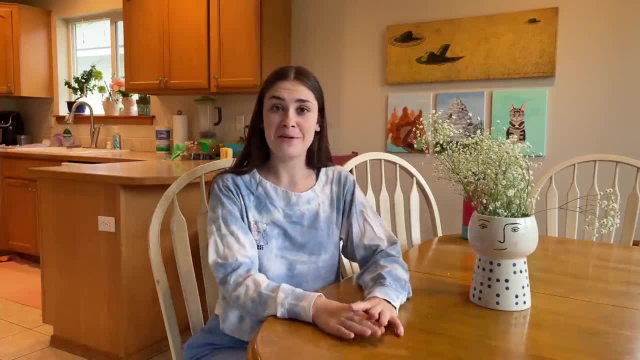 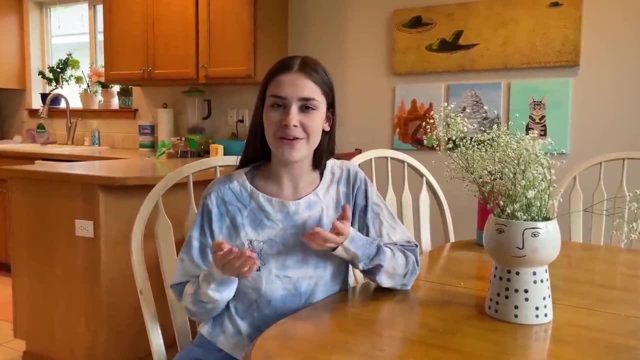 and I ended up somehow- I don't even know how- doing these big ball gowns immediately. So I was able to get a sewing machine and I watched a lot of videos on YouTube, kind of like this one, and figured out how to sew. 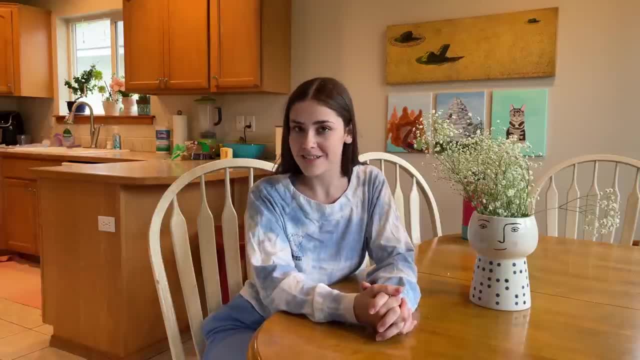 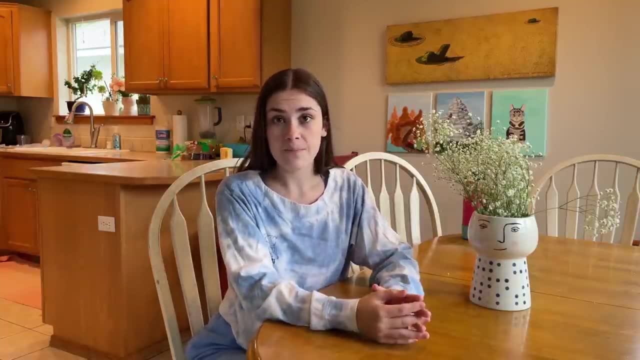 I also have always used my own patterns because it's a lot easier to customize, and I do that by draping, And I actually didn't learn how to drape until a year later, because I did not have a mannequin, until a year later. 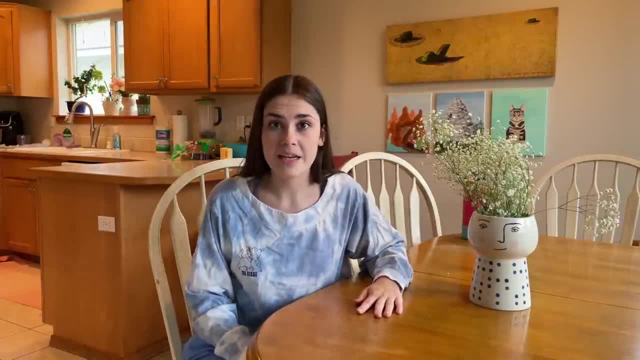 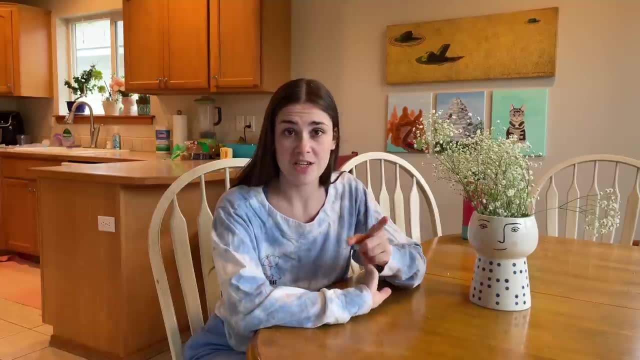 So the very first year of sewing, I didn't have a mannequin. Actually, maybe it was the first, like five or six months, because I started sewing in June and I got my first dress form on my birthday, which was October 4th. 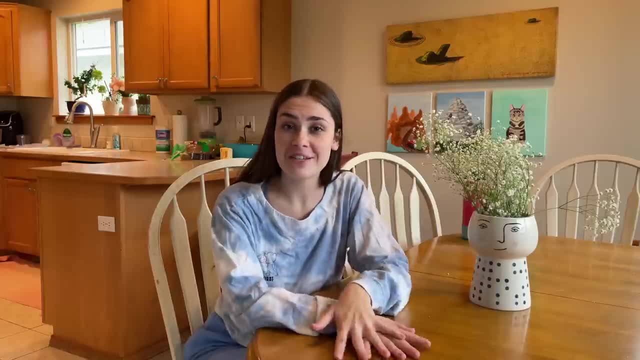 So, whatever the math on that is, But you can do it too. If I can do it, you can do it. So today I want to show you all of the supplies I use and I want to show you where to get them. 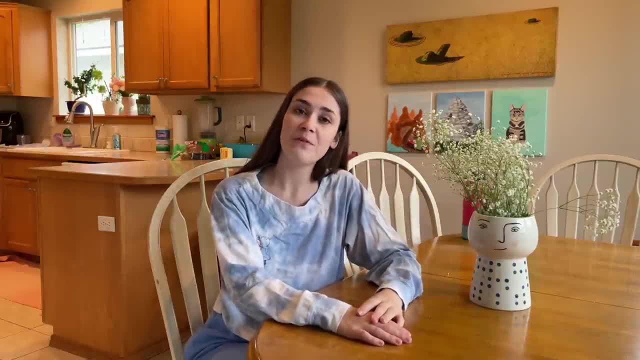 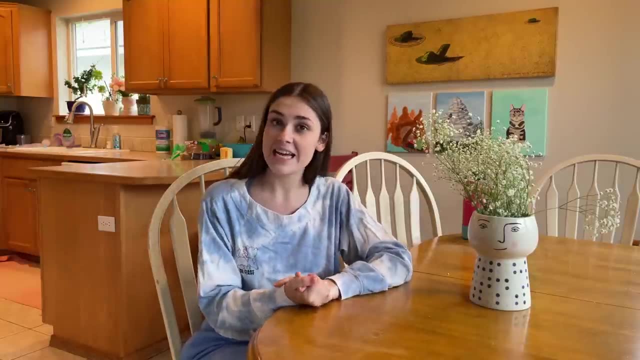 Almost everything that I talk about will be linked in the description below if you want to get it for yourself. And I promise that sewing is not as hard as people think it is, and I'm going to teach you how to sew, And at the end of this video. 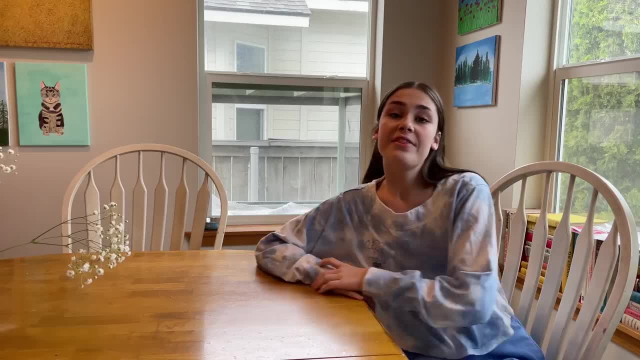 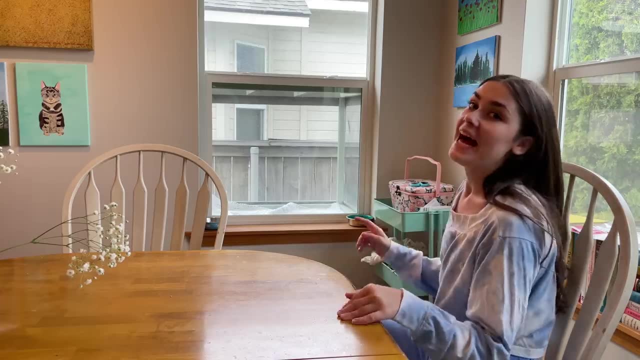 I hope you feel a little bit more confident in learning how to sew yourself. I think that we can all agree: the most important thing you need for sewing is- can you guess it? A sewing machine. I keep my machines over in this corner because there's nowhere else for me to keep them. 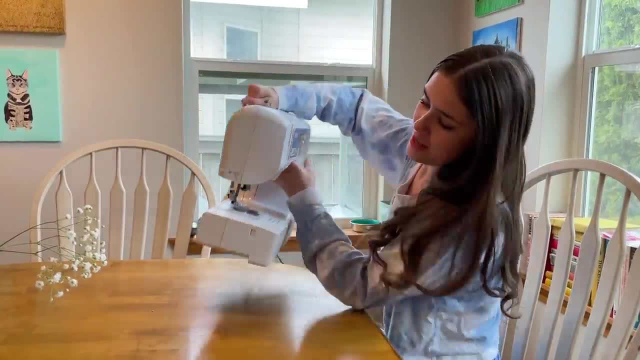 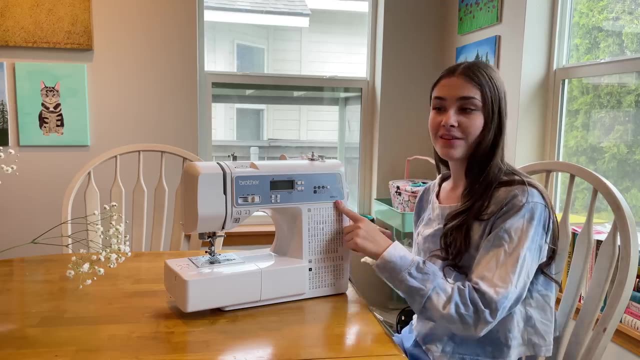 So every time I sew I gotta pick it up. bring it up here. This is my sewing machine. It is a Brother XR9550.. I got this on Amazon. I believe it's about $200 or $250.. I've had it for over a year. 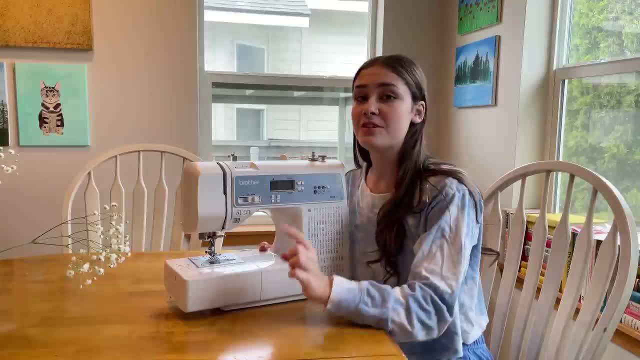 and it works very, very well for me and I recommend it to everybody. So this will be linked in my description box below, And I really think this is a great machine to get if you're a beginner, or even if you're not a beginner. 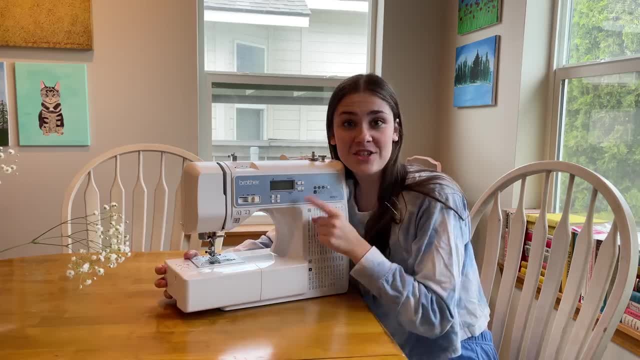 It works very well for me. It gets the job done, So I think that you should get this. Obviously, you don't need a sewing machine. I mean, if you really wanted to waste the time to hand sew, you could hand sew. 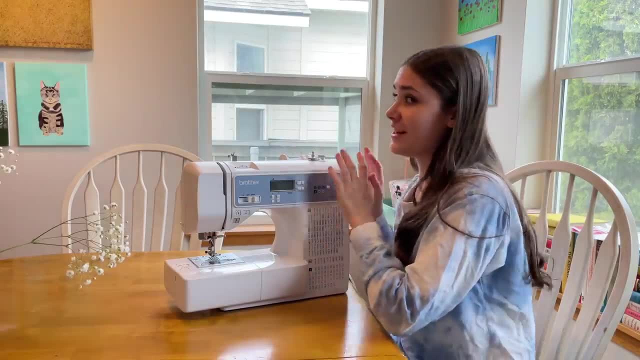 but I don't really recommend hand sewing. I think you should get one of these And I will show you how to work this later, but let's move on to the other things that I have Now. I'm gonna tell you right now. 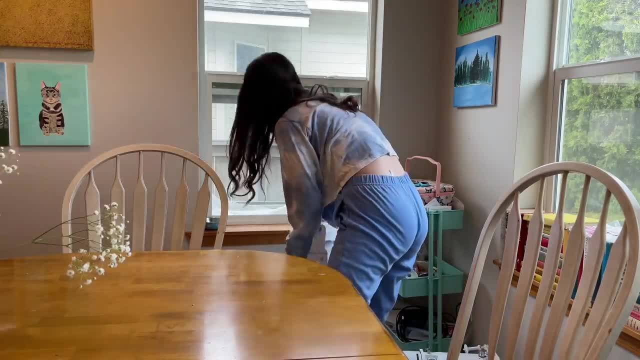 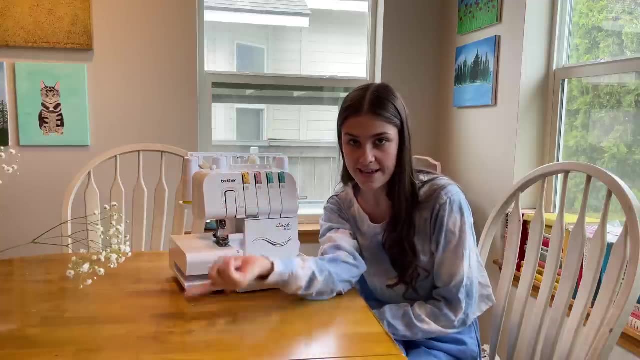 you do not need a serger. I do have one, but I do not have one for the very first year that I learned how to sew. I started sewing, like I said, June 2020, and I think I got this around February or March of 2021,. 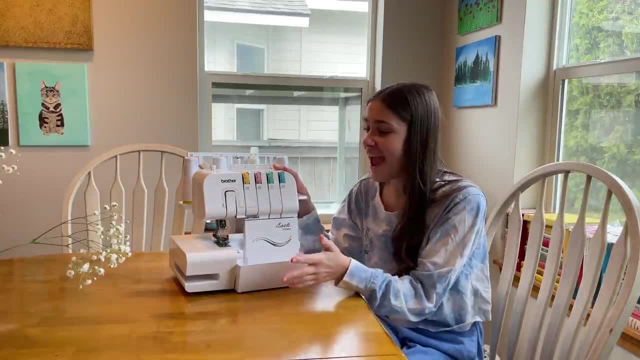 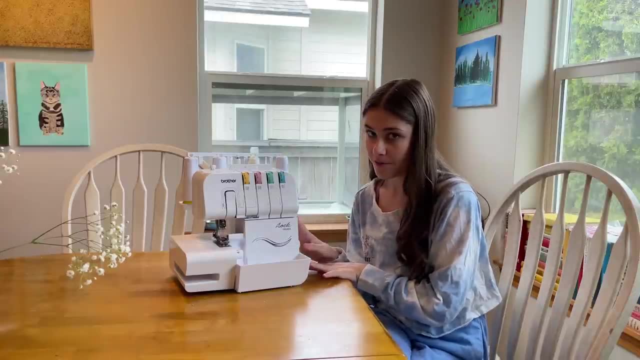 and I used my TikTok creator fund money to get it And I have the Brother Lock 1034DX. This also has worked very well for me. So if you wanna feel more professional, you can get one of these linked below, but you really don't need it, I promise. 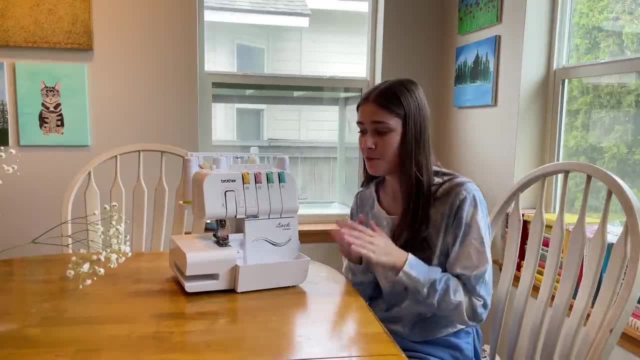 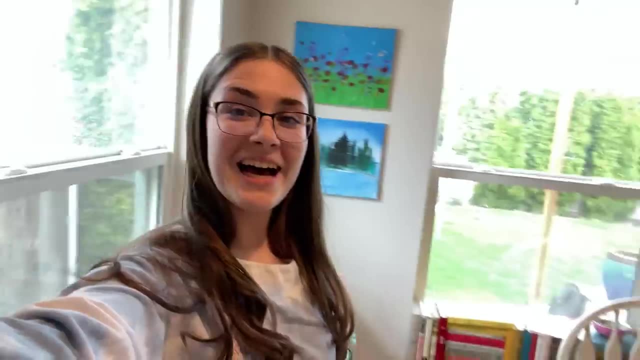 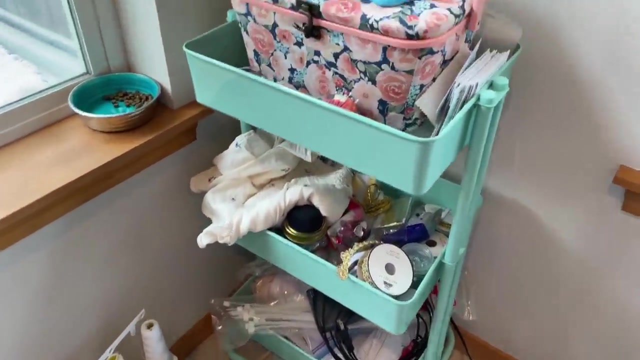 You can find ways to make dresses without having a serger to finish the seams. Now I'm going to take you over to my sewing corner and show you up close and personal, my little organization tool. Organization is definitely a key part of sewing. 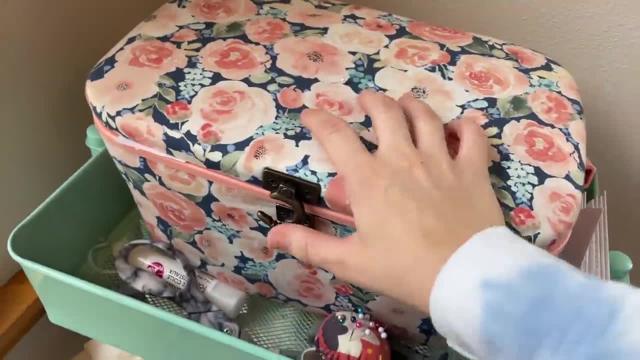 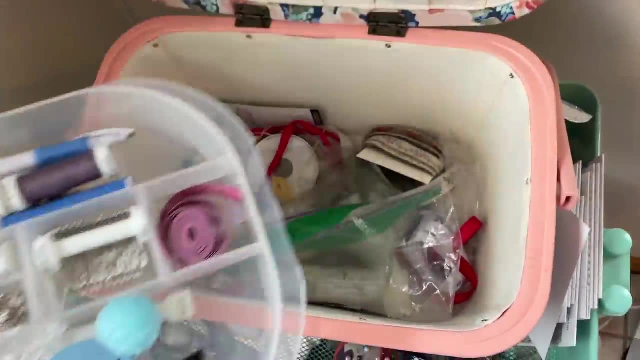 I use this little sewing box- I think it's from Walmart- every day And I just have some threads. This is not all my thread, It's just a great place to keep everything, And then there's also space under there. You're gonna need some fabric scissors. 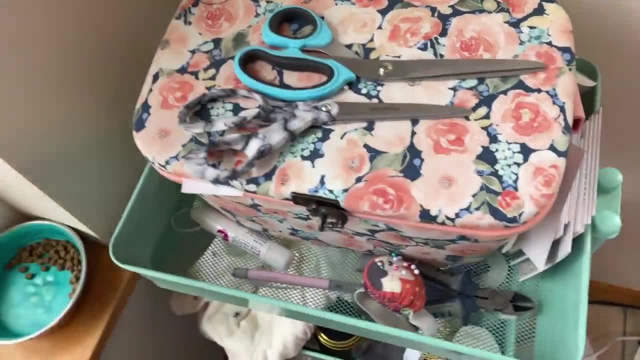 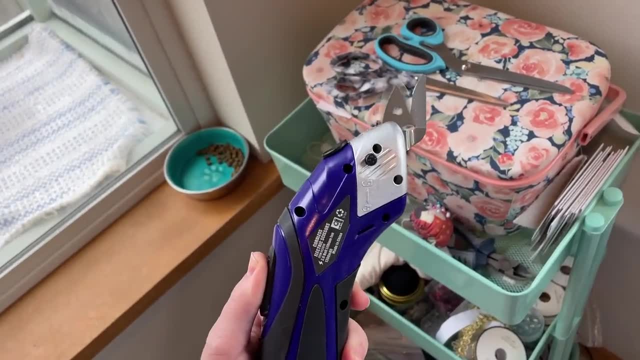 I have a few. I have this one, This one, I also have this. I really recommend They're electric scissors. Listen to this. That's moving so fast you can't even see it. These are a life changer. They're so easy to cut fabric with. 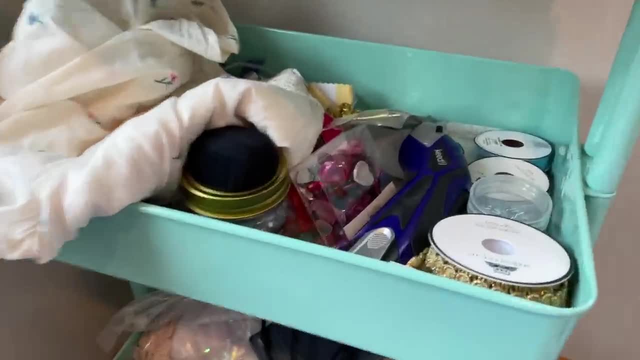 They're linked below. Rest of this I don't think you really need. It's just some of the things I've been using. I have beads, grommets. You kind of need these if you want to do a corset. 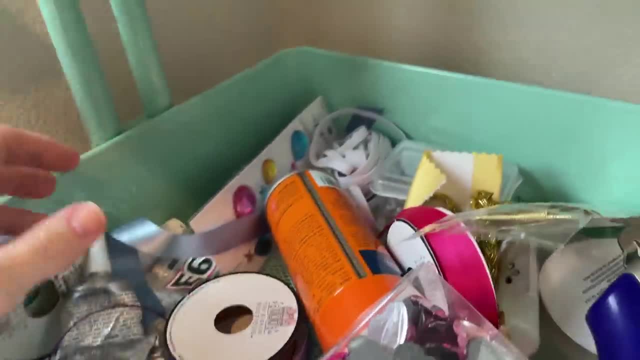 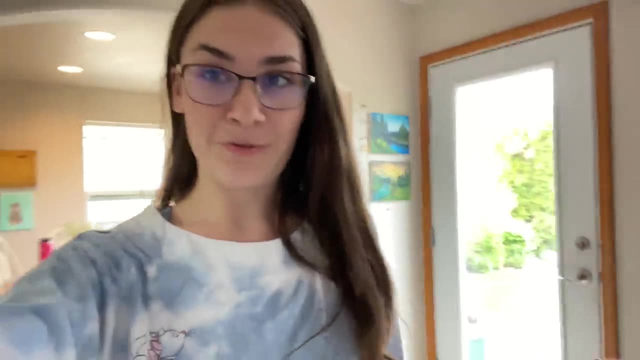 But other than that, I just have some things. I've been working on all my ribbons and stuff, And if you think that's all of my sewing supplies, you're wrong. I have a whole sewing closet as well. Now don't freak out, because you're about to see. 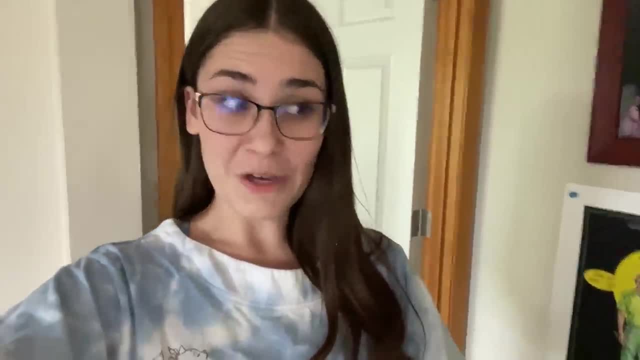 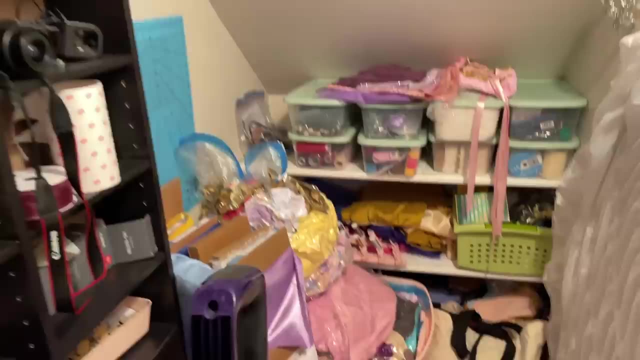 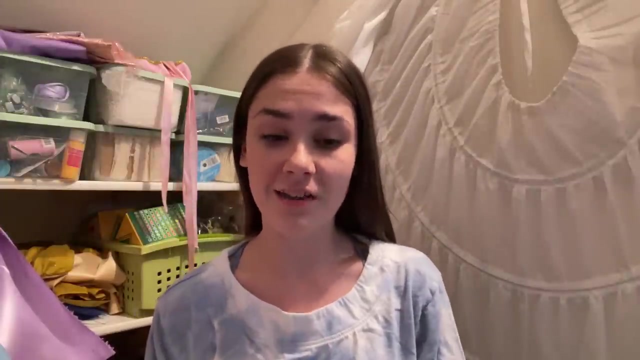 a messing sewing closet, But I'm moving in a month, so it's just holding on for dear life until I get my sewing room Under our stairs like Harry Potter. I have this monstrosity of sewing supplies. Up until Christmas, I was in California at college. 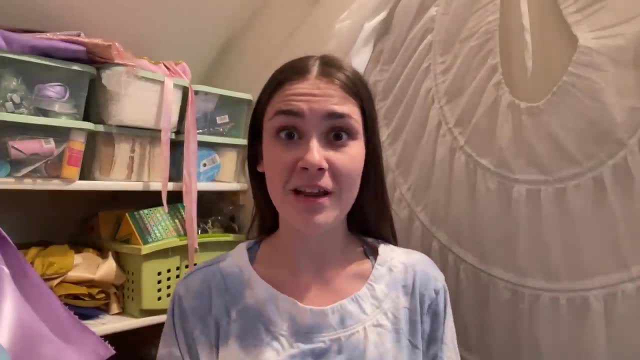 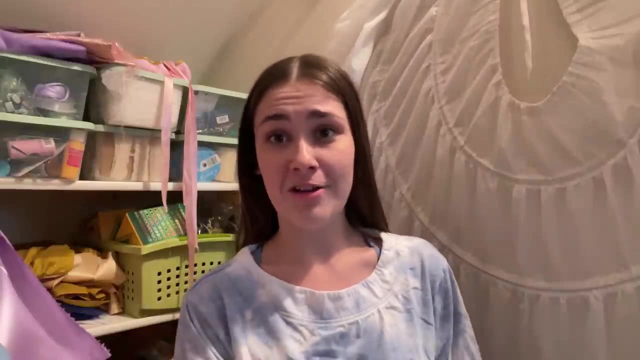 but I made the decision to leave because my sewing career has been doing so well. So I moved back home temporarily and my mom cleaned out our whole closet under the stairs for me to use as storage until I was able to move out. So this is where I've been keeping all of my things. 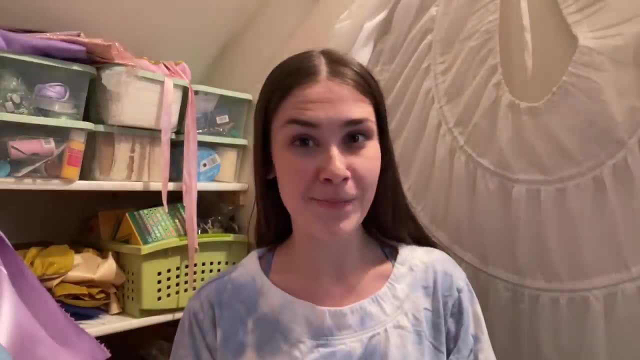 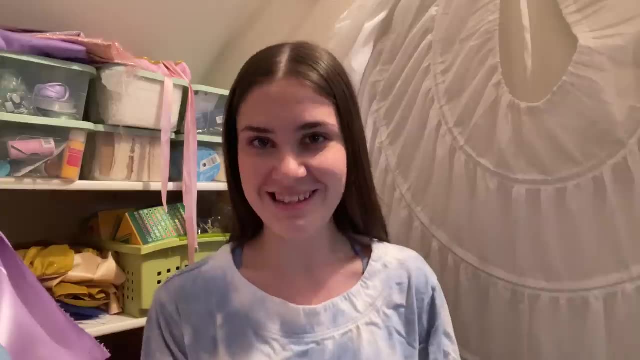 You can see that I try to be organized but it does not work because things just build up quickly. when I'm sewing I just kind of shove things in here. But let me take you on a little tour of this closet. First and foremost, I have my mother load of dresses. 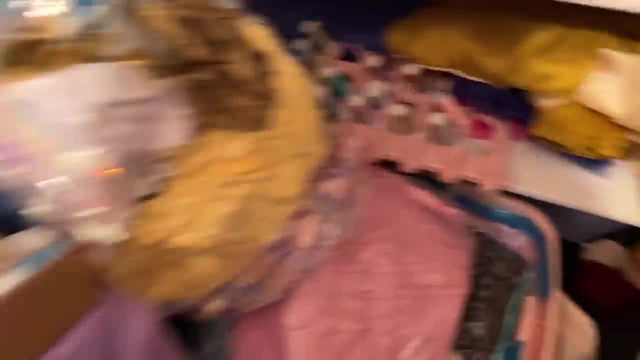 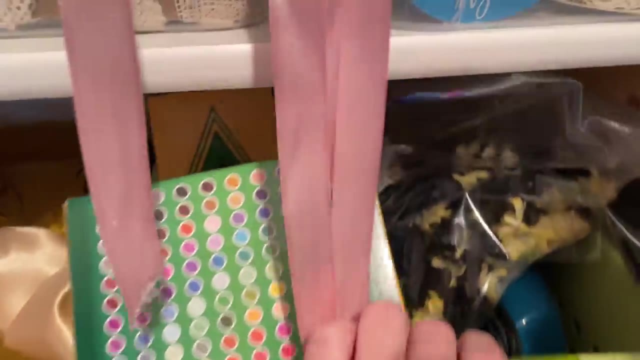 These are all vacuum sealed. I have some bolts of fabric and more bolts of fabric- Fabric down there and fabric in this bag and in that bag, fabric right there- And then this is a miscellaneous. I'm not going to tell you exactly what these markers are for. 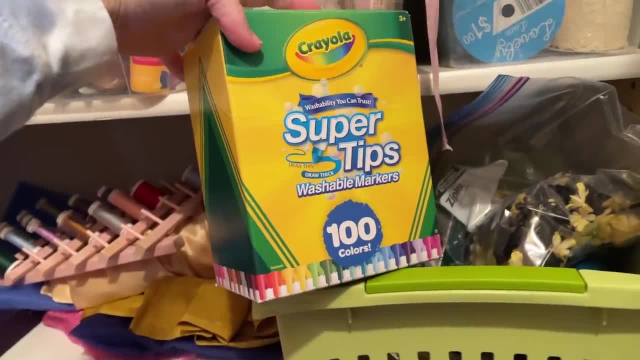 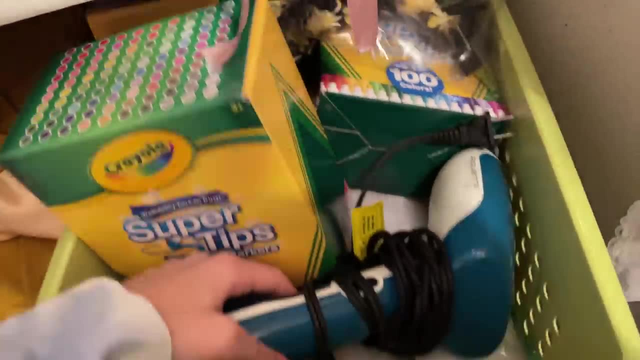 but I'll let you know that I'm making a dress out of them, And if you grew up watching Disney Channel, you're going to know what dress I'm making. Other than these markers, I have a steamer and some miscellaneous things. 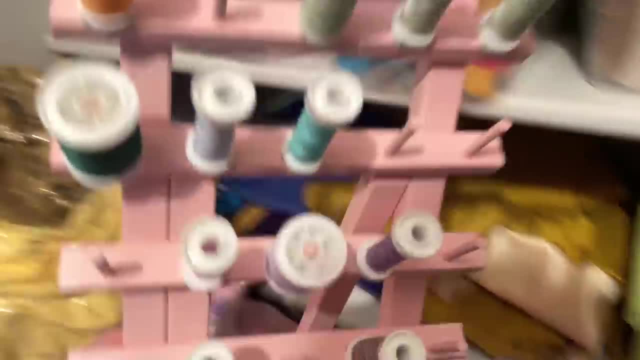 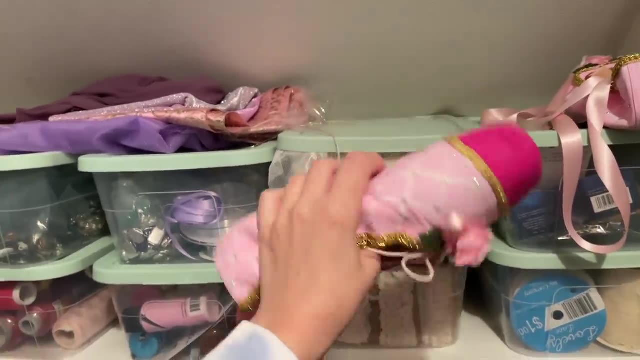 I have my thread right here. I want to hang it up, but not until I move. And these: if you watched my 12 Dancing Princesses dress that I posted last Friday, you'll recognize these. If you haven't watched the video: 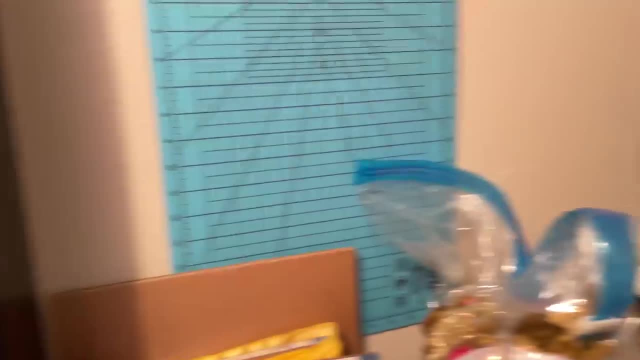 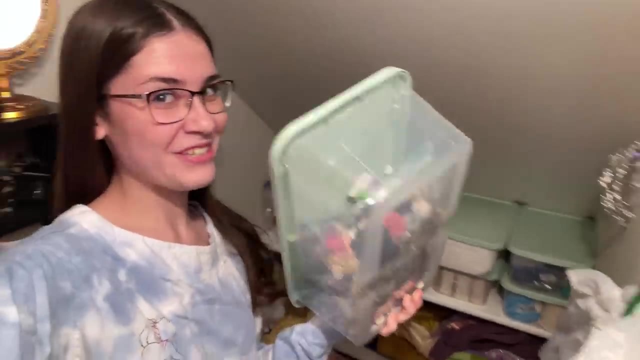 go watch it right now because people are loving it. But the favorite and best part about this closet, I think, is what's in these bins. Firstly, I have- oh my gosh, this is heavy- My button bin. Let me show you the inside. 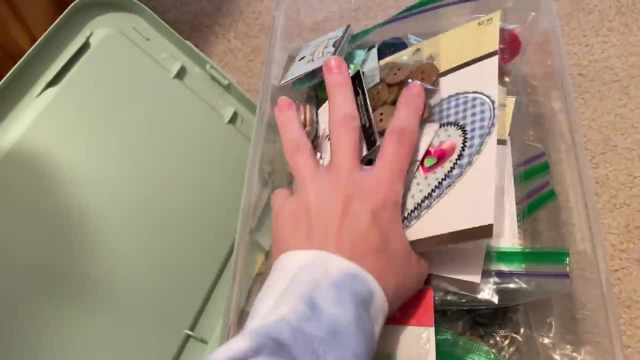 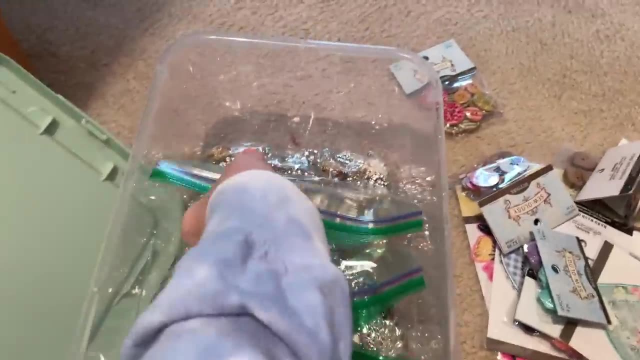 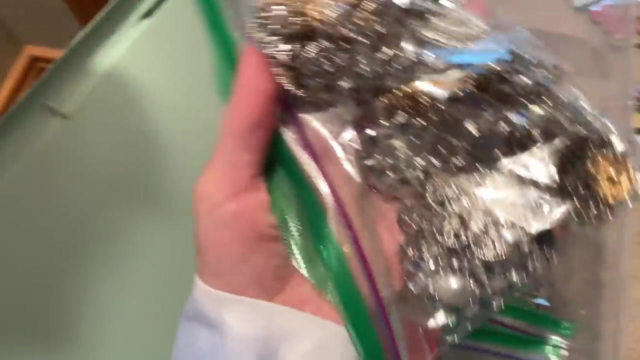 In. this is where I have all of my buttons and some patches. These are just normal buttons: Buttons, buttons, buttons, some cool buttons And then my favorite, like beautiful rhinestone-y buttons. So I have literally hundreds of them. 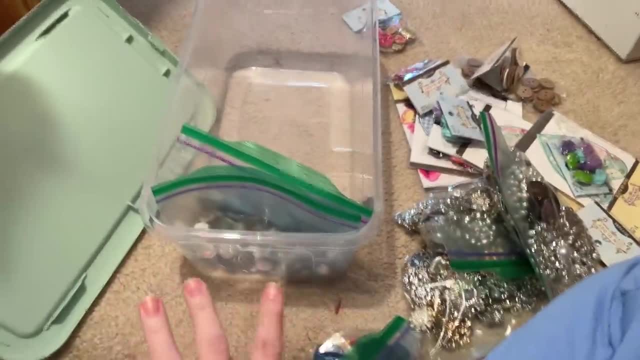 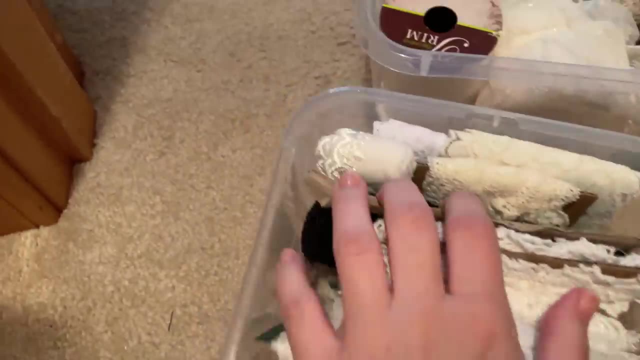 Aren't they so pretty? You don't need this many buttons, but I have this many buttons. These three bins are actually my very favorite. They have all of my laces that I've wound up onto these little cardboards. Now we're going to move from that to this behind me. 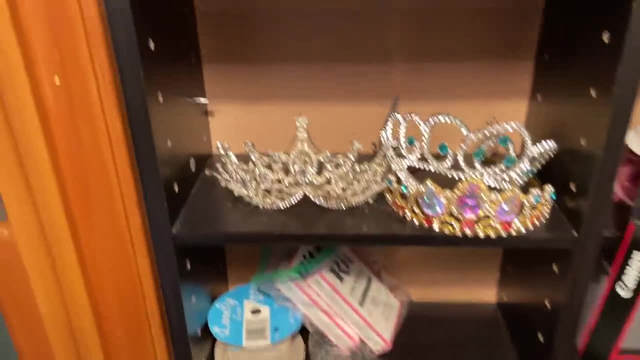 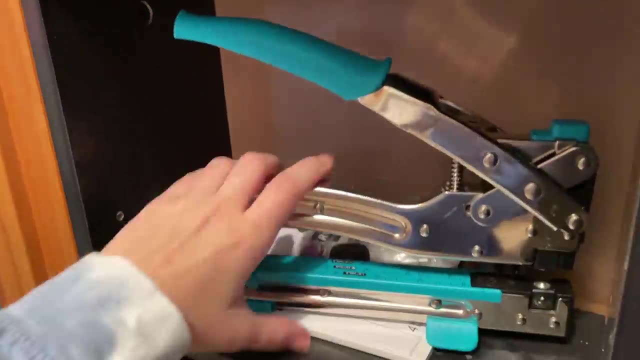 These little shelves I'm able to store random things. I have my tiaras, my dye, this great costuming book and just random things. This is what I use to put grommets in, Kind of punches them down. 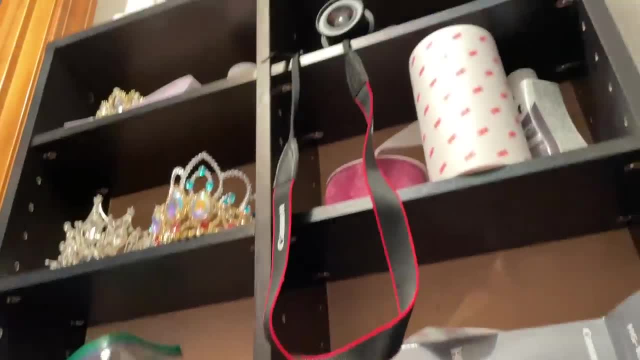 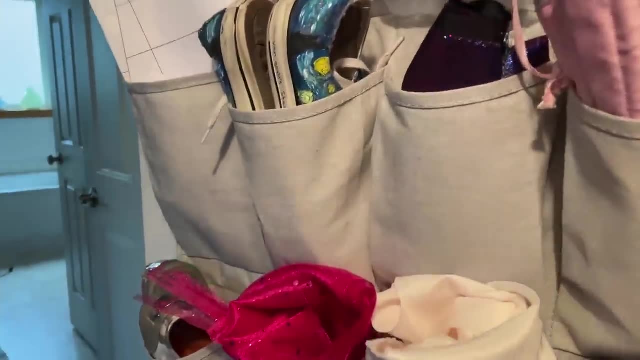 Really just random stuff that I don't know where else to put. And then I use this shoe rack, but I just stuff random fabric scraps and things that I'm working on. So if I ever am working on something with fabric, I'll stuff it in here. 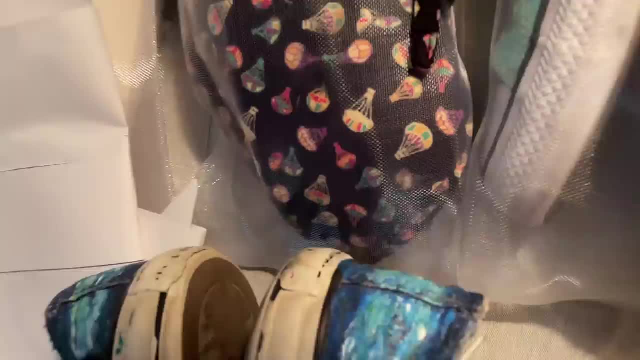 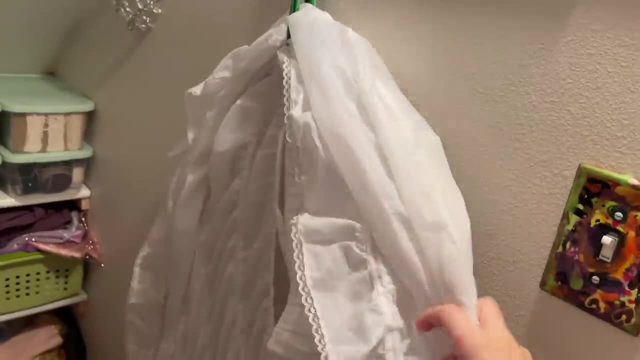 I have some other things too, like some pattern pieces. But yeah, this is my sewing closet Because I thought you might just be curious of where I keep my stuff. We can't forget my hoop skirt. It's really easy to hang and it just goes right here. 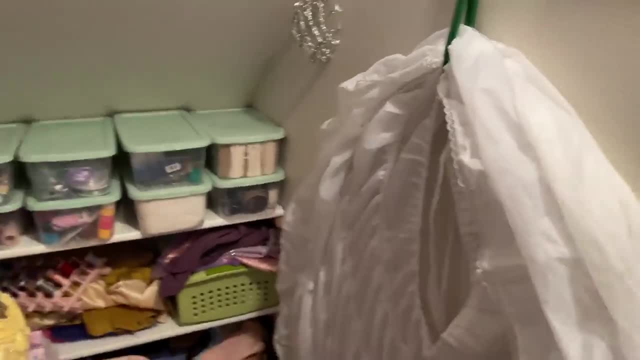 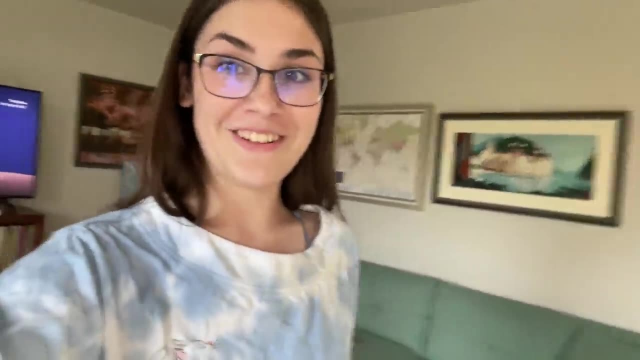 People always wonder where I get this stuff. It's from Amazon and it's linked below, as well as a lot of other stuff. Okay, so I'm sure that you probably have PTSD at this point from seeing that mess of a closet. So now let's go sit down and we'll talk about where to shop for all the sewing stuff. 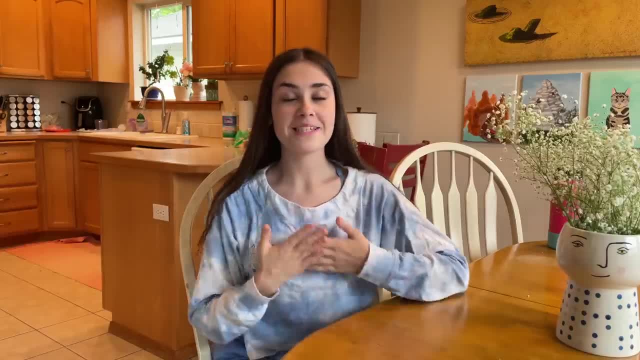 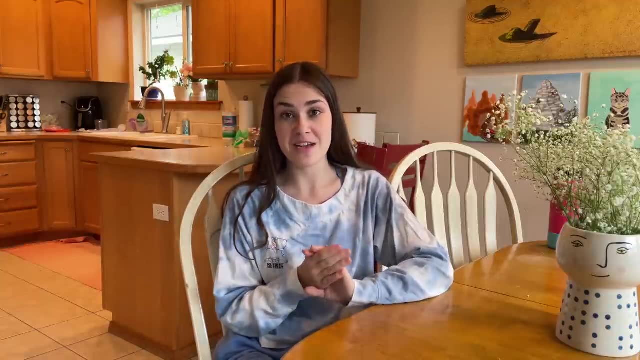 and what my favorite stores are. If you're looking for fabric, the best place that I recommend will be Fabric Wholesale Direct. This is an online store with incredibly cheap but great quality fabric. I use it for so many projects, especially in the beginning of my sewing journey. 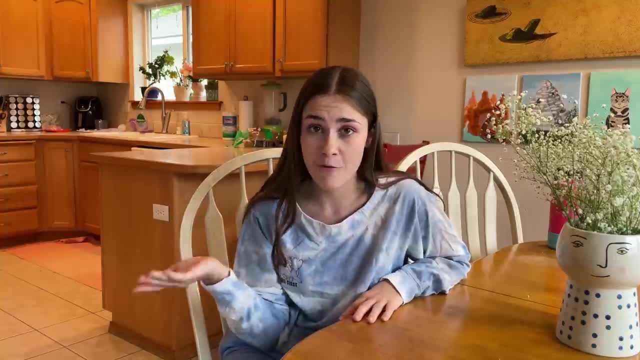 when I didn't have a large budget, And I also think Joann's has some great options. It is a bit pricier, But you probably have a Joann's where you live and you're able to pop on over and get what you need. 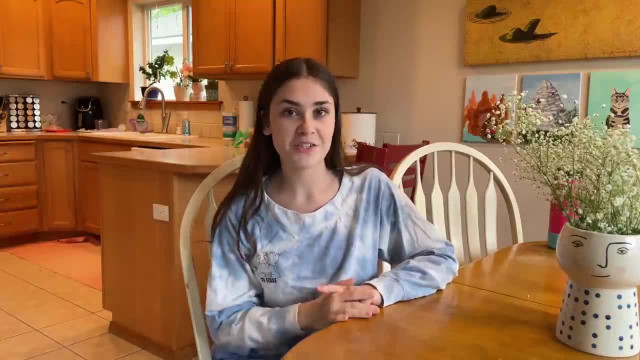 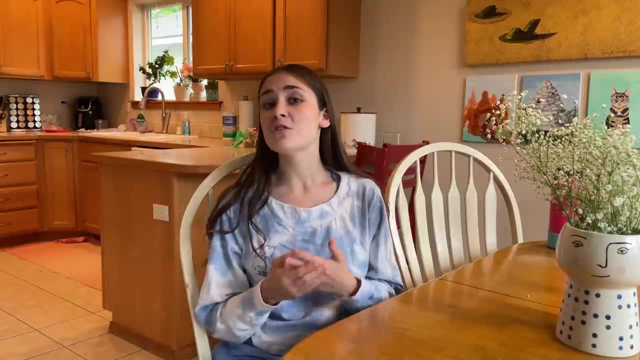 Etsy is also a great place to find more specialty things. This is where I bought the color-changing fabric for my Aurora dress, as well as some great laces. So those are pretty much where I get all of my fabric. Let me know if you have a different fabric store. 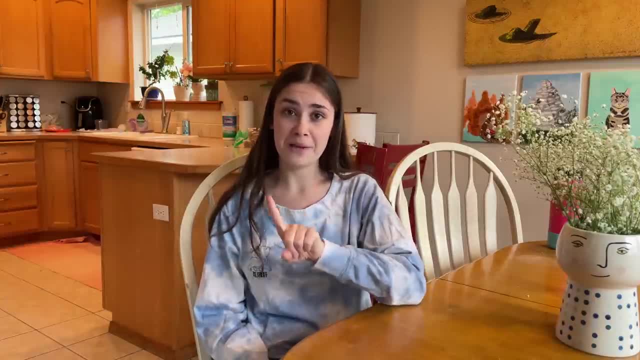 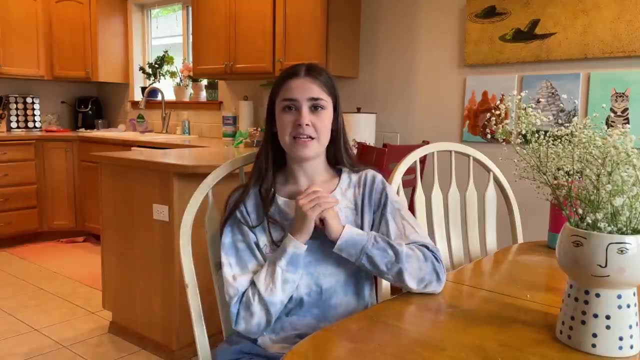 I just know that where I am, the only fabric places I have are Hobby Lobby and Joann's. Other than that, I don't know. I have to do all of my shopping online, which is totally fine too. It's just a little sketchy, because sometimes you don't know if it's going to be what you're thinking of in your head. 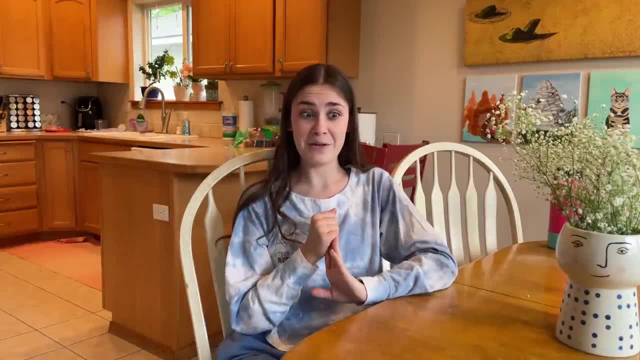 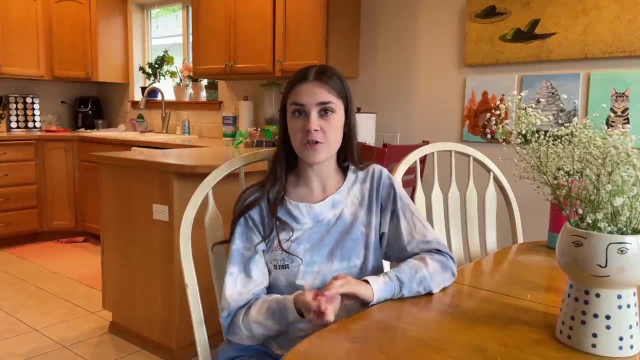 And there's a lot of times where I'll order something online and I'll get it and I'll be like that's not what I wanted. But Fabric Wholesale Direct. I really recommend them if you're first starting out, because they have a huge, huge selection of fabrics for a great price. 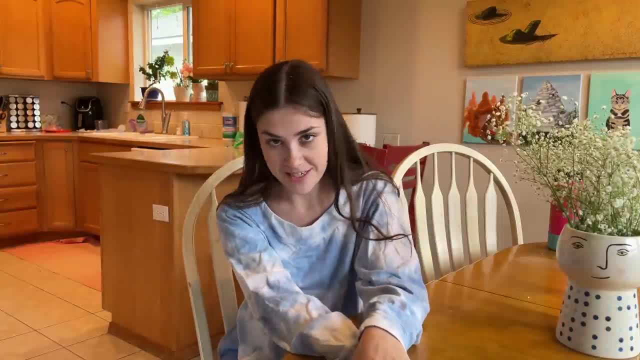 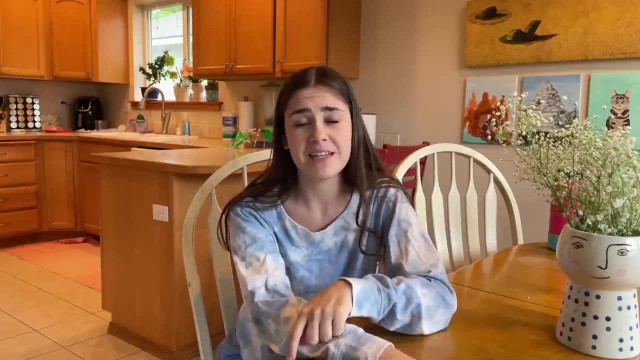 If you need a dress form, I have a few different recommendations. The best beginner one I could recommend- I can't remember exactly the name of it, but it is adjustable- and you can get them at Joann's Amazon, I think the one I have linked below is from Amazon, if I remember correctly. 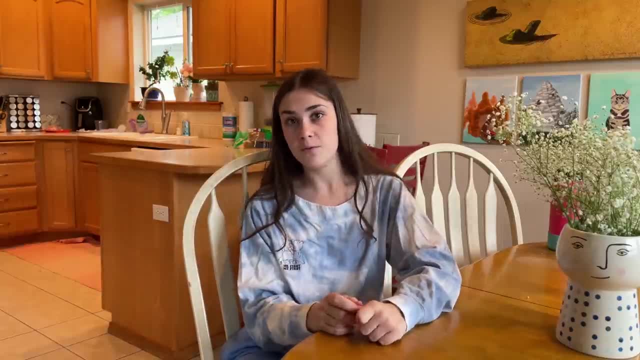 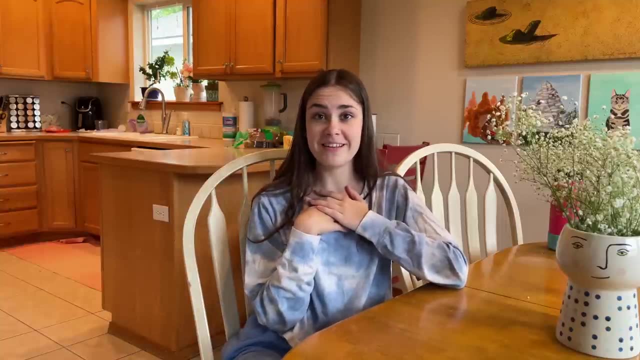 But it's very cheap- I think it's $100 or $200- and it's adjustable, So you can make it exactly your measurements. I use one of these adjustable ones for probably about two years, And then, when I went to college, I bought myself a really, really nice one from Royal Dress Forms. 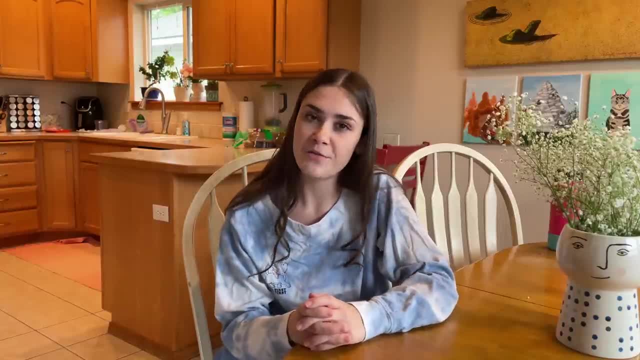 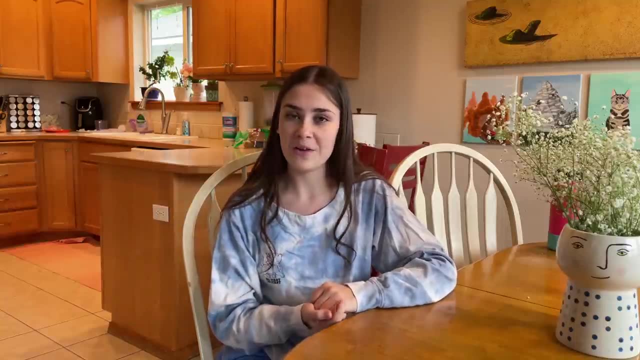 I'll admit it's very, very expensive, But I personally do think it's worth it if you're wanting something very nice, very good quality and if you're really serious about what you do. But I really recommend that you just start out with one of the cheaper- $100 ones. 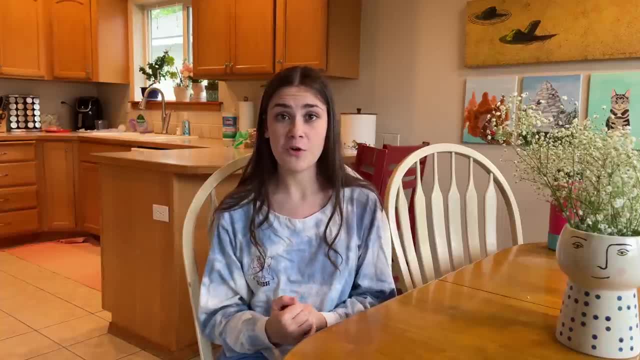 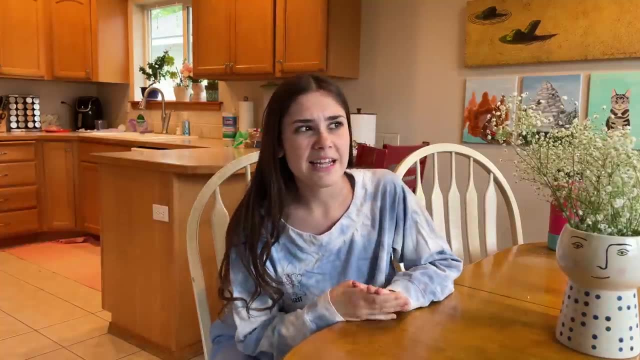 And, like I said, you can buy one of those below and I will show you what my dress from looks like And I'll kind of show you how you use it. Finally, the only things that I can think of that you might want to buy now are like patterns. 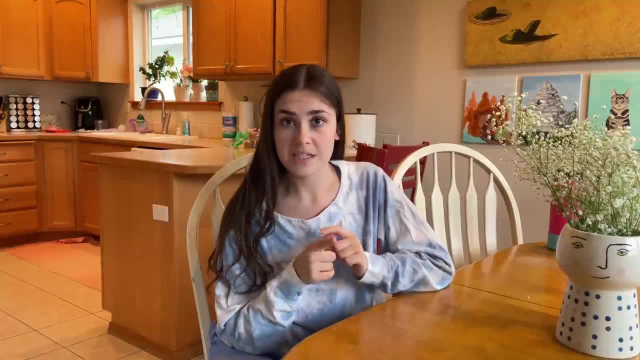 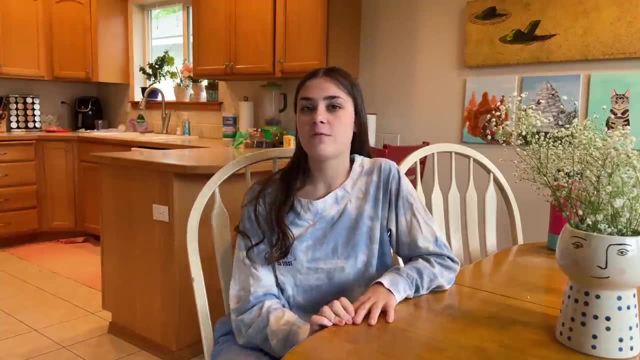 If you don't know how to make your own patterns- Mood Fabrics- They have a whole website with so many hundreds and hundreds of free patterns. that are great if you don't know how to make your own. And, of course, you can also buy patterns. 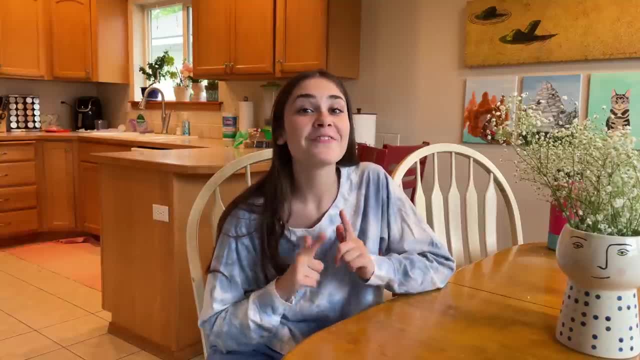 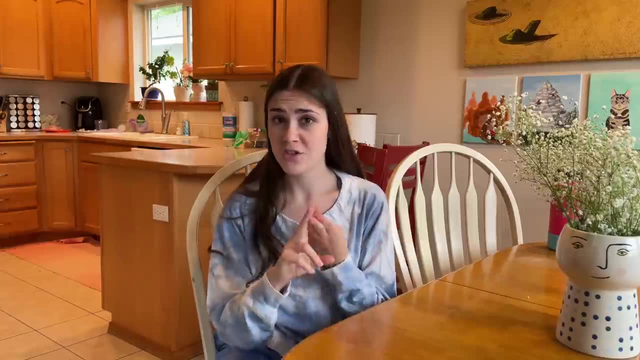 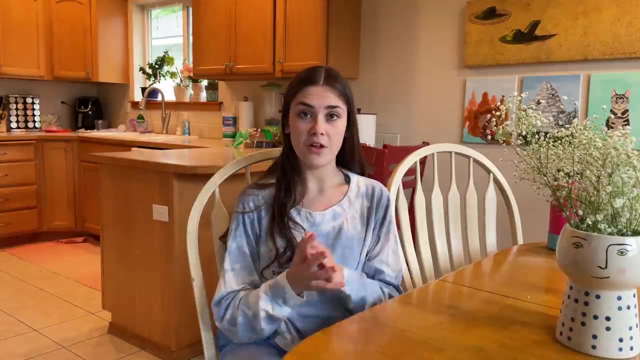 I would always check Mood Fabrics first, because they are free. And then, of course, we have our miscellaneous things that you can get at any craft store, such as thread, scissors, measuring tape, markers, pins. That's all going to be at Joann's Amazon, Michaels Hobby Lobby, wherever you look. 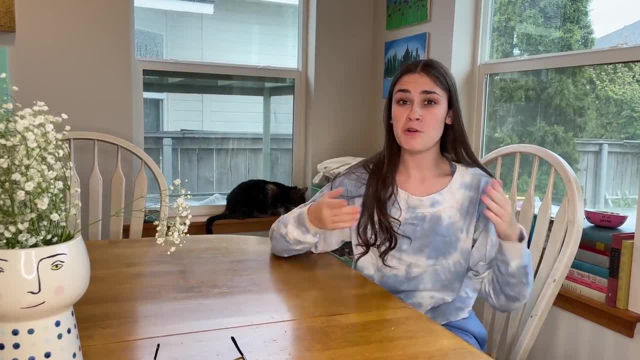 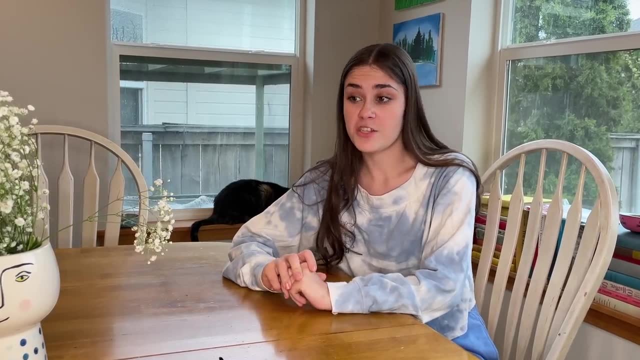 I want to keep this video pretty simple, so I'm not going to be showing you a super in-depth tutorial of everything I do to sew. But I do want to show you how to work, thread, turn on and sew with a sewing machine, And I might show you how to make a skirt. 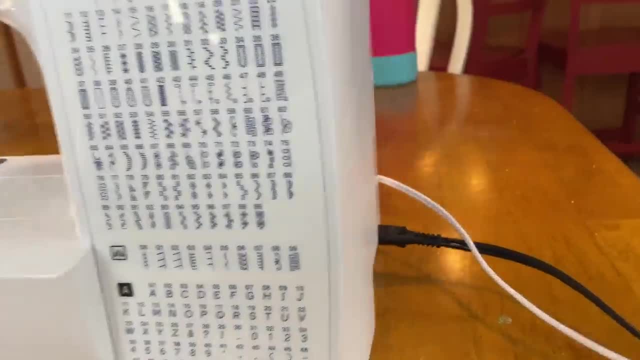 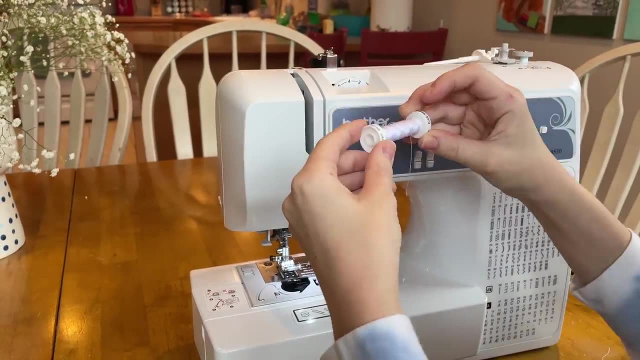 I'm going to start with the sewing machine. I have turned this on and it is threaded, but I will show you how to thread it first. You're obviously going to want a spool of thread And up here you're going to have a place to put your thread. 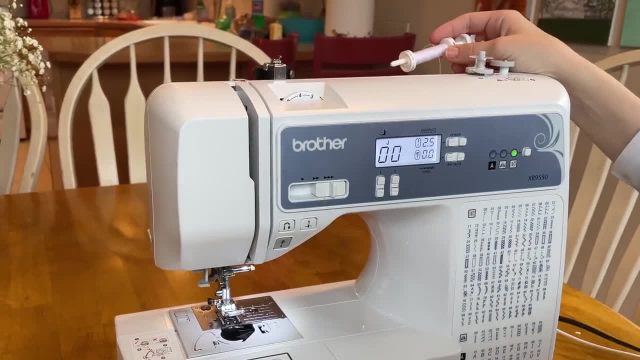 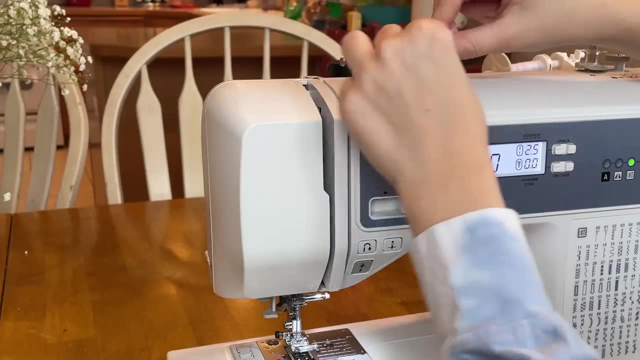 So put it on like that, And then your sewing machine should have a cap And you put that on so that it doesn't go anywhere, And then we have the thread. You're going to put it back here and it's going to loop around. 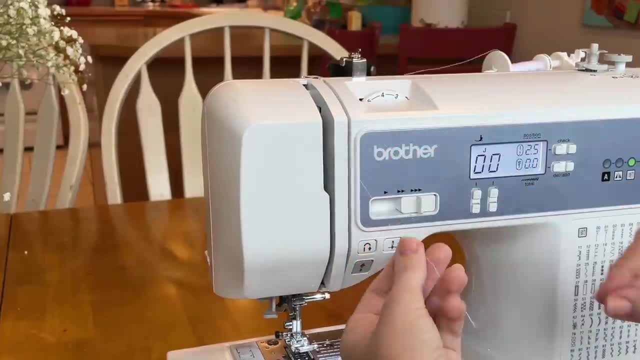 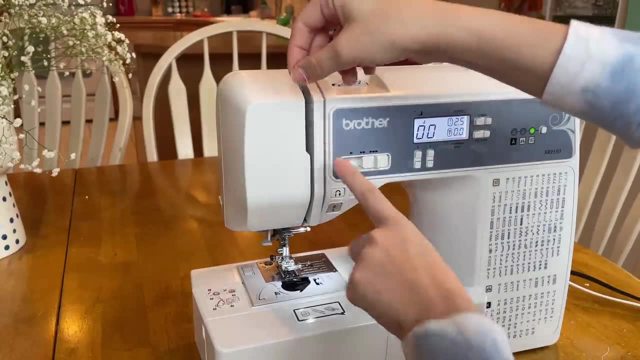 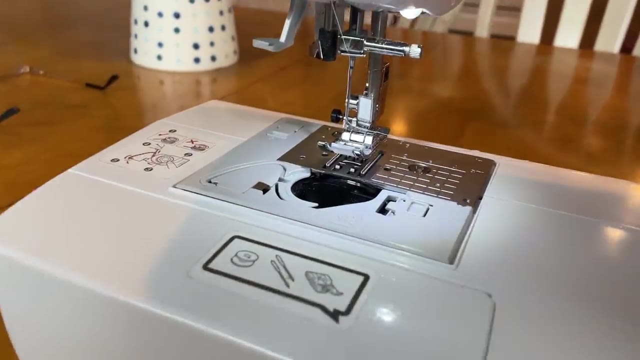 And you should have this kind of thing, And you're going to pull the thread down up around like that. There's a little metal hook inside, Pull it back down again and then you will thread it through the needle. I know for a fact that I was not very good at teaching that. 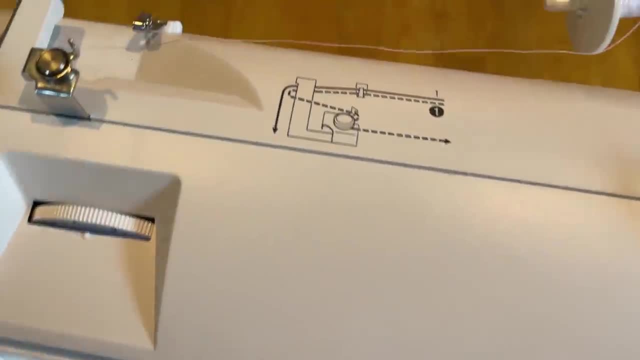 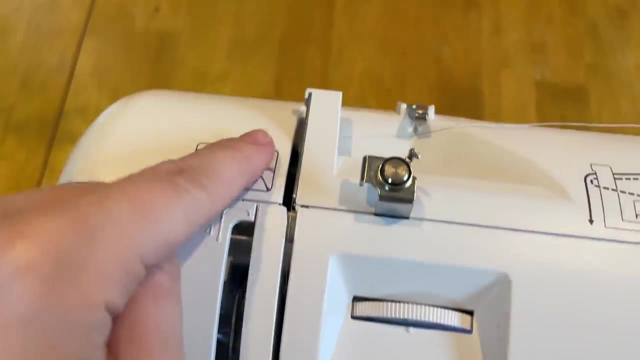 So let me show you up close. There are directions on the sewing machine So it's pretty self-explanatory. So the thread, at least on my sewing machine, goes around this thing. You're going to bring it through this little hole. 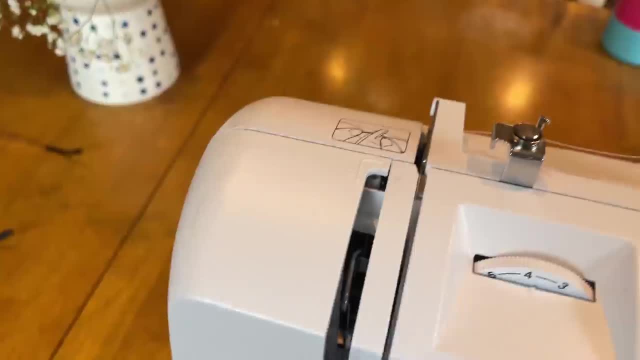 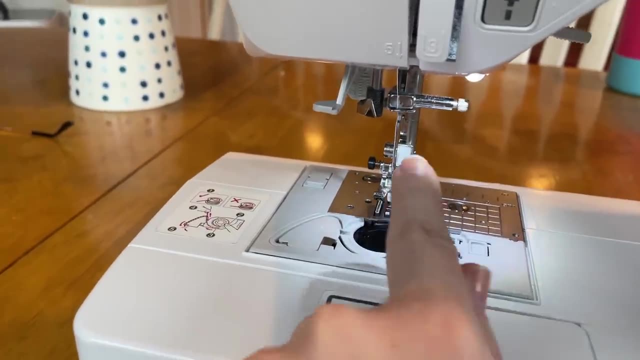 Around. See it says three. You go around and up And then you'll see there's a little metal thing in there. So number four will go around again. Bring it back down, Number five down here. Put the thread behind that little hook. 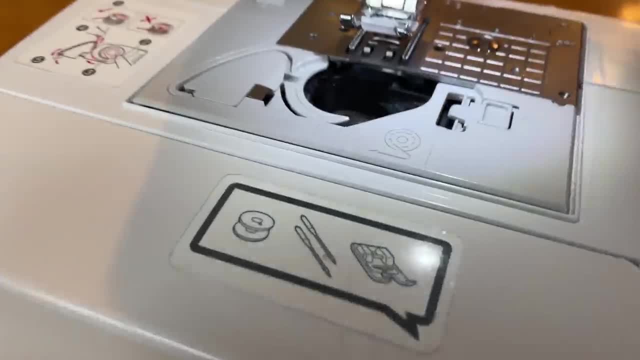 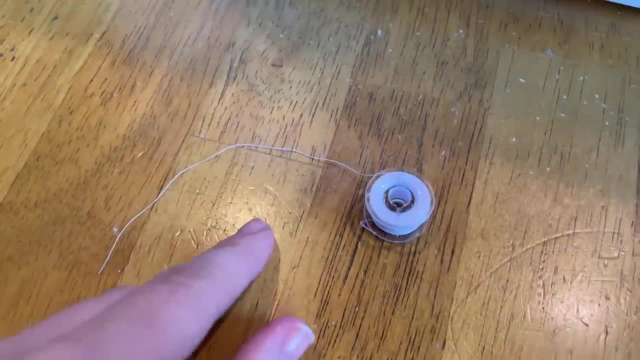 And then you're just going to put it through the needle hole. of course you'll need a bobbin. that's this right here, and you thread it up here. when you put the bobbin in, you want to make sure that the thread is going counterclockwise, and i'm just going. 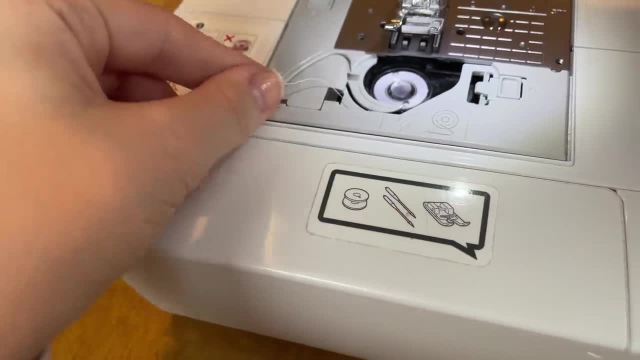 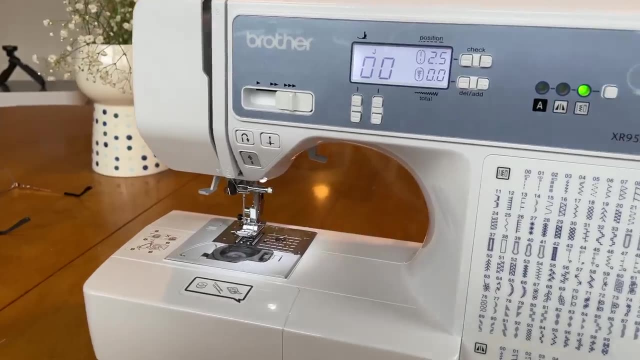 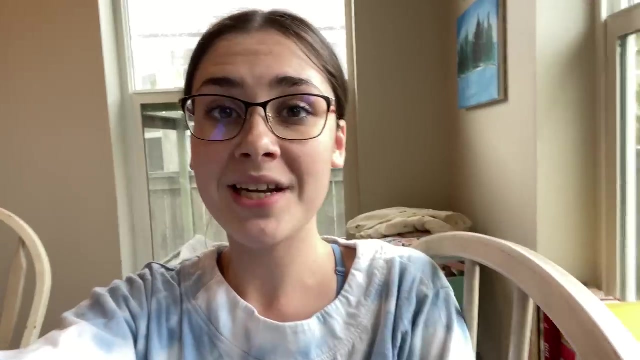 to pop it in like that: take the thread and, through this diagram right here, go like that and then we'll put the cap on once you get your machine threaded. it's pretty easy to do. you really can just start sewing and i will show you a little scrap test. i'm going to keep this as simple and 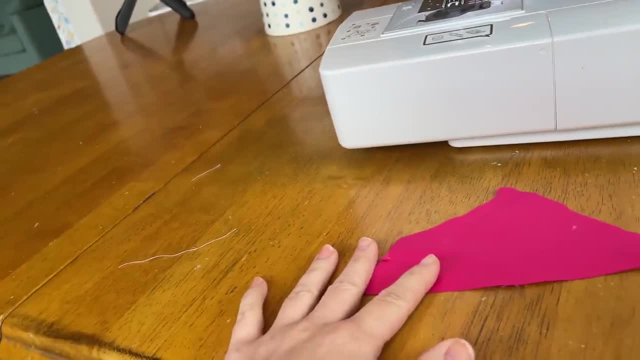 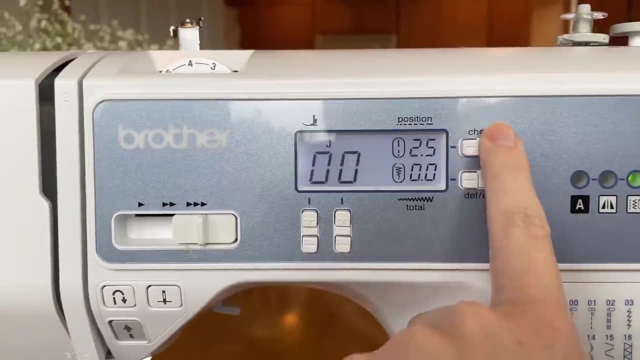 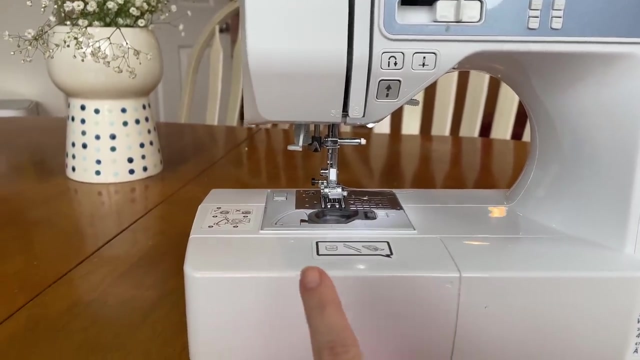 basic as possible. i'm just going to be sewing with this scrap piece of fabric and right now we're going to do a straight stitch which is number zero on this machine. here you can change the stitch lengths, and so that means like how long it will be with each stitch to make the machine start to go. 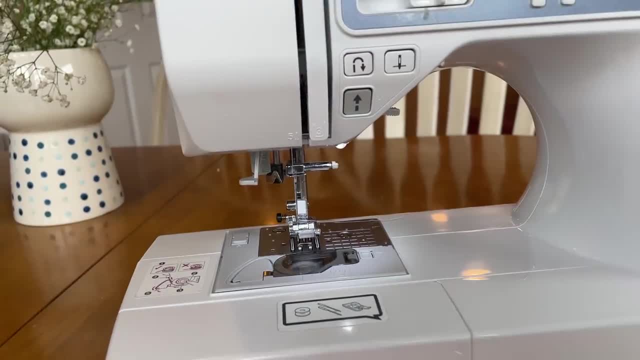 we're going to push our foot down on this petal and just have the fabric under here for today. i'm going to start sewing with this scrap piece of fabric and i'm going to start sewing with this piece of fabric and i'm just going to be sewing these two pieces together with your pieces. 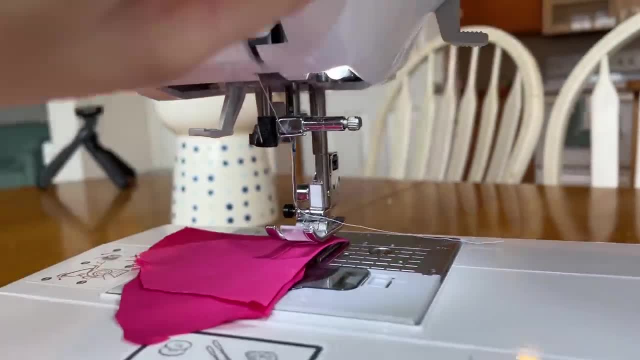 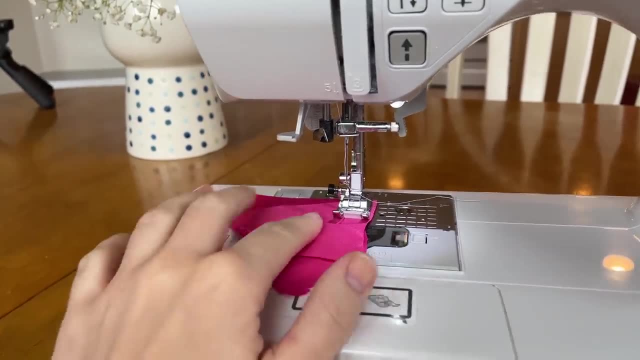 together. you're going to put it under the foot and there's a little knob back here. you're going to put that down and that will make this go. the machine will not run unless this foot is down, because it's a safety hazard if it ran whatever. so with the pedal that i just showed you, i'm 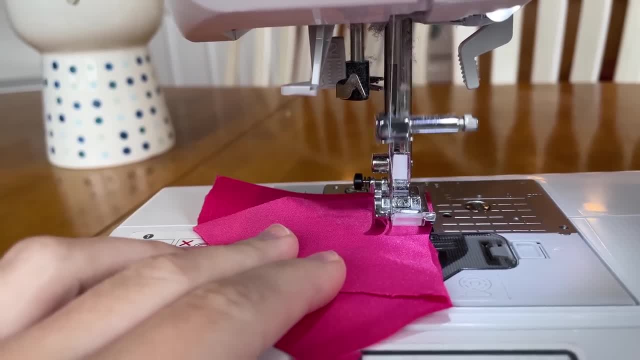 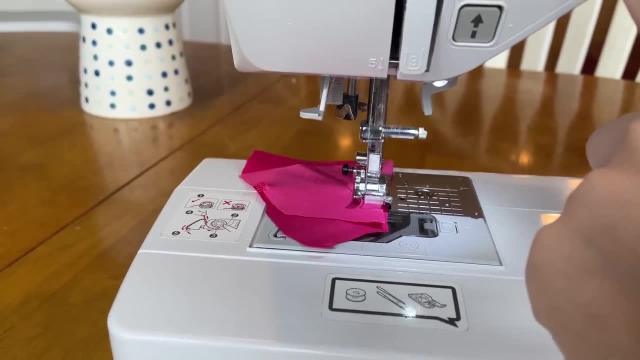 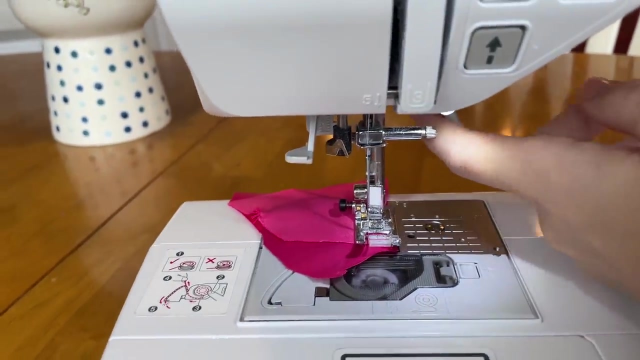 going to take my foot and press it down and it's going to start to sew up here. you can dictate how fast it goes. so this is as slow as it goes and if you want it to go fast. so i just sewed the two pieces together and i'm going to lift this bag up, pull it out and cut off. 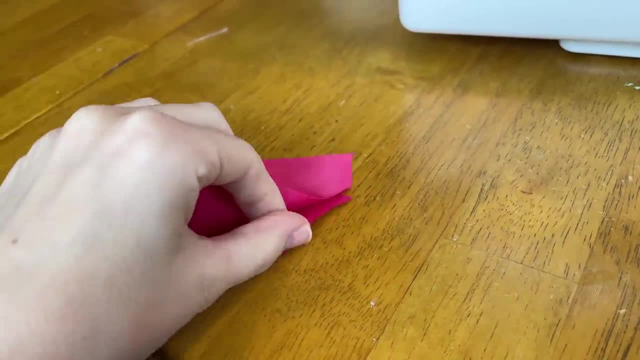 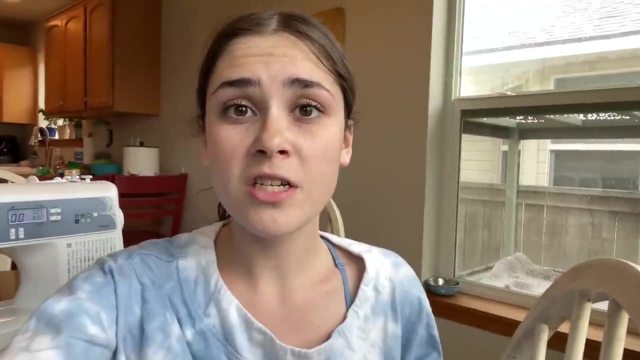 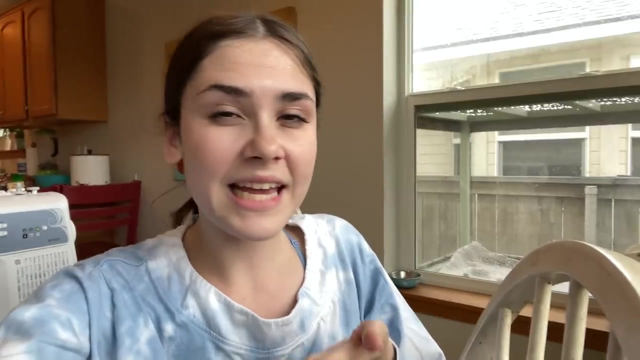 the threads. there you have a stitch sewn and if you open it up like this, you have pieces that are sewn together, and that's really as basic as it gets. there aren't many other stitches that you will use on a day-to-day basis other than the straight stitch and, i suppose, occasionally. 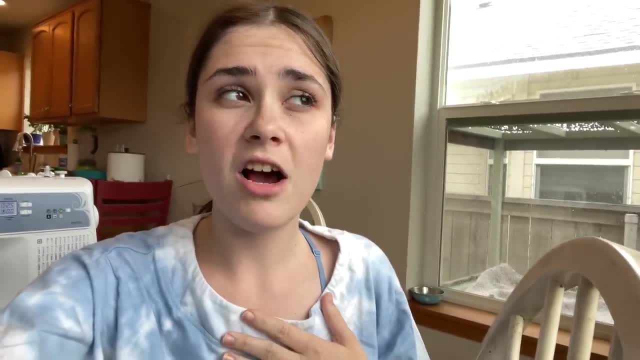 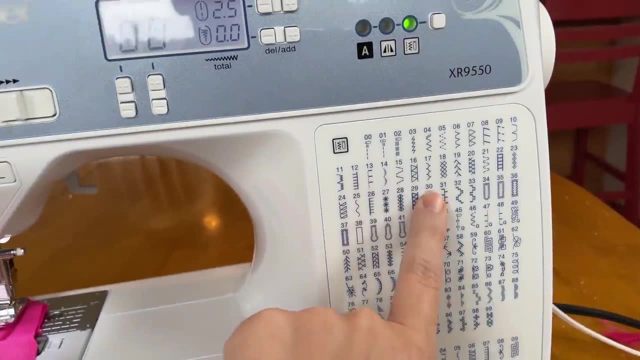 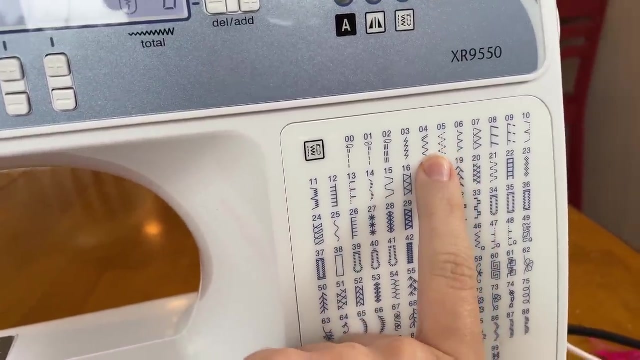 a zigzag stitch which i can also show you. but i honestly couldn't tell you what other stitches i use, ever other than those two. but if you want to use any of these fun stitches, or even the zigzag one, you just put the corresponding number up here. so if you want to do a zigzag which you're able to, 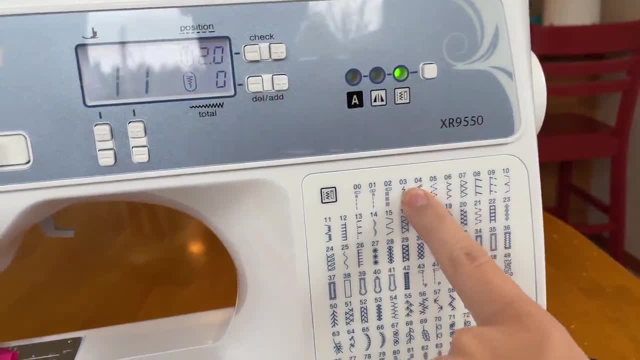 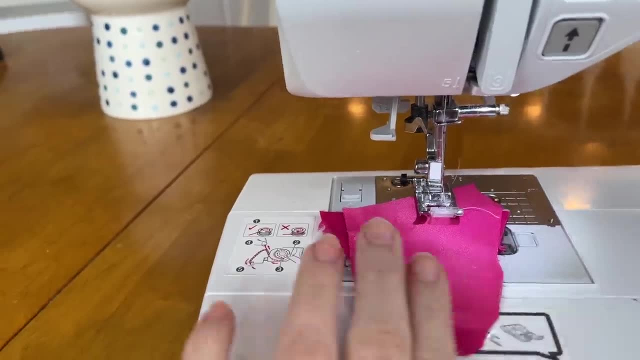 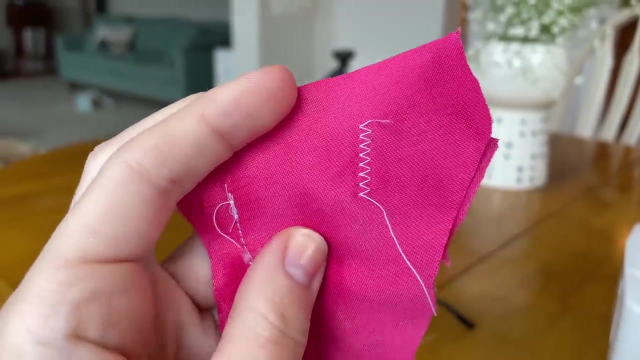 use. instead of a serger you can use a zigzag stitch on the edge of something, so that's number four, and then you can also change the length of it. so for that one, you'll see that i'm going to make sure that the needle zigzags, so you can get a nice little zigzag going and it turns out looking: 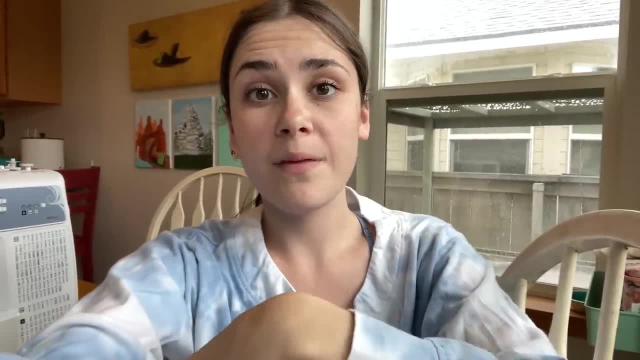 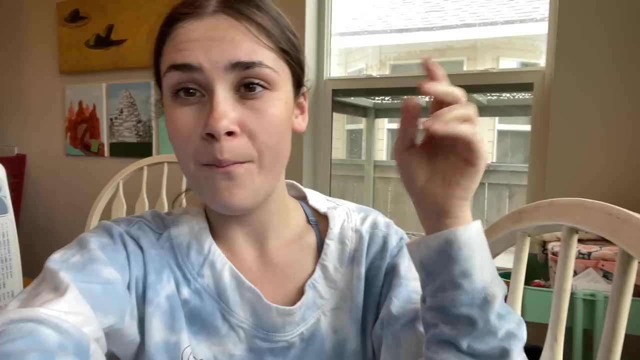 like that. that's all i'm going to show for the sewing machine today because, like i said, i wanted this video to be very basic and before i leave, i wanted to show you two more things: which is my dress form and also a basic way to get you started on doing big ball gown skirts. this is our music. 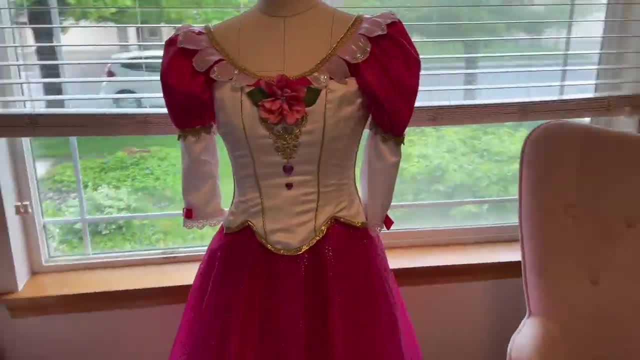 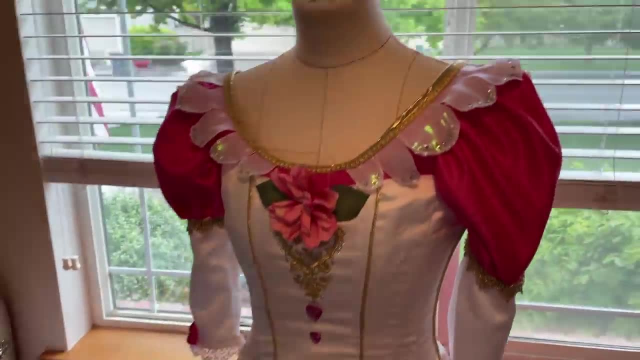 parlor and for now, it's where i keep my dress form. i always have something on display. right now, i have my 12 dancing princesses dress out and, as you can see, i have my 12 dancing princesses dress out and you can see, this is my mannequin. it's quite nice. underneath it's a bit squishy and you're able to. 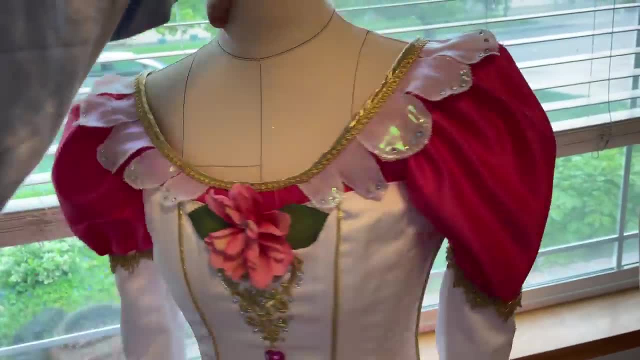 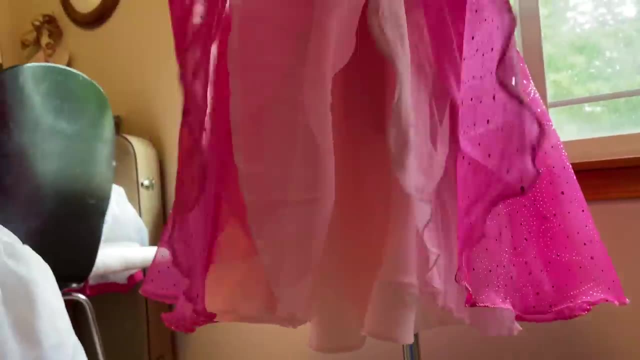 do so many things with it. i love this mannequin. like i said, it's from royal dress forms, but the adjustable ones are just as good. now, what i want to talk to you about are all of the skirts on the dress form. all of these skirts are what are called circle skirts, which is exactly how it. 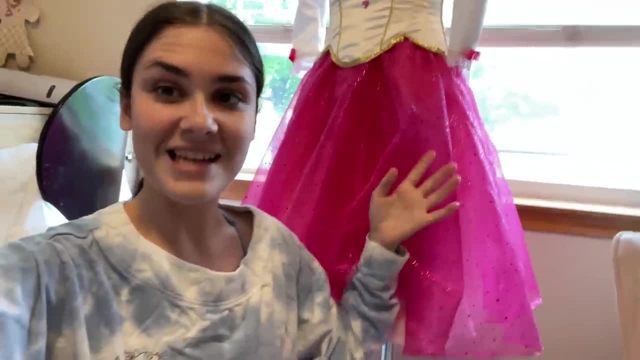 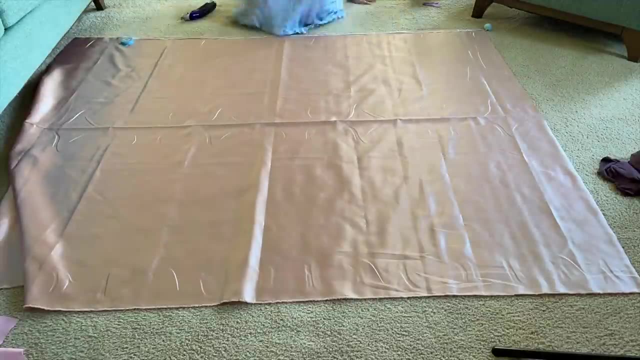 sounds. it's literally just a circle with the waist cut out. i will put a time lapse of myself cutting out a circle skirt and then i'm going to cut out a circle skirt, and then i'm going to cut out a circle skirt. so you can see what it is: a circle, and the measurements for this are quite. 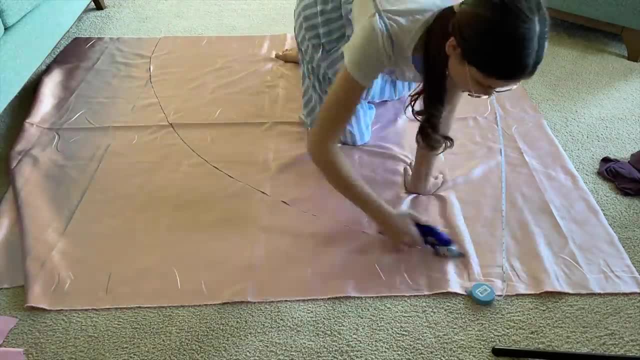 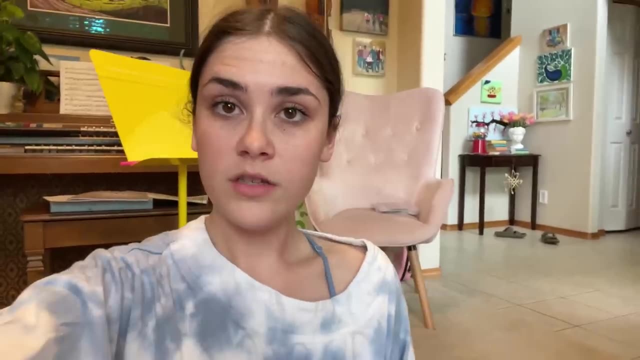 easy. i always do the biggest waist radius possible so that i can gather it up, and then the larger radius for the outer edge will just depend on how long you want the skirt to be. so if you want to make a very large ball gown, such as the video that i showed you with the time lapse, i will use the. 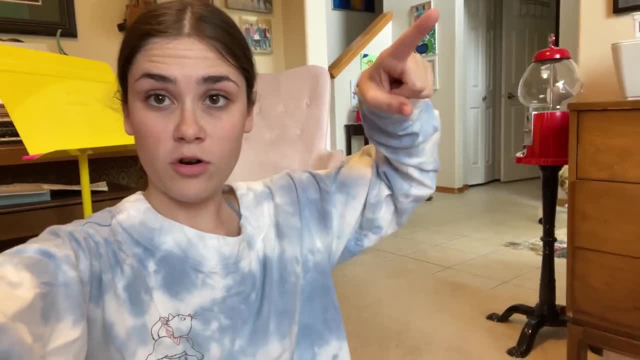 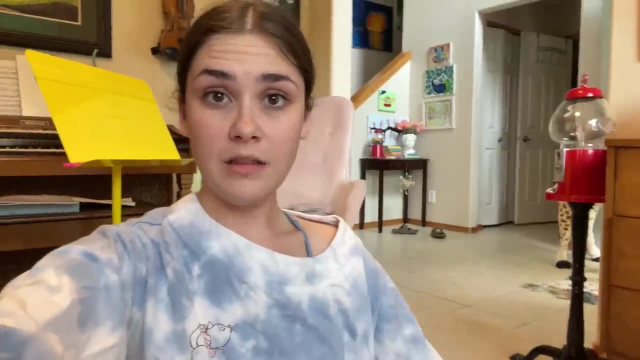 entire 60 inch width of the fabric and cut a circle that is 60 inches wide and then the waist radius. i will make 15 inches so that i end up having a full circle skirt. and then i will cut a 45 inch long skirt and a very large waist to gather, because this isn't really a very in-depth. 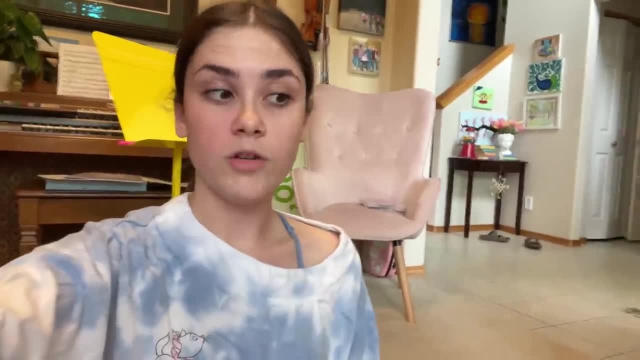 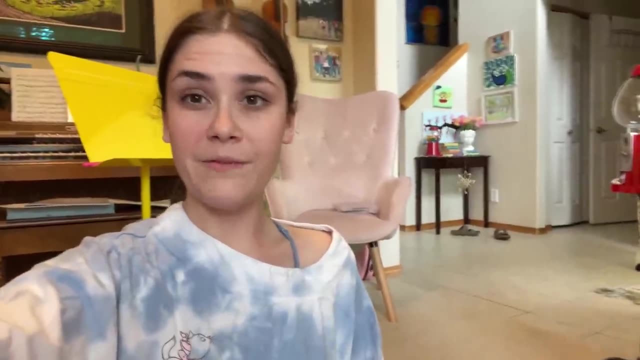 tutorial video. i suggest searching up on youtube how to sew a circle skirt, because there's going to be a lot of better tutorials out there than what i can make. i just wanted to kind of explain my way of doing things, because i wanted to make a video telling you guys how i do everything again.